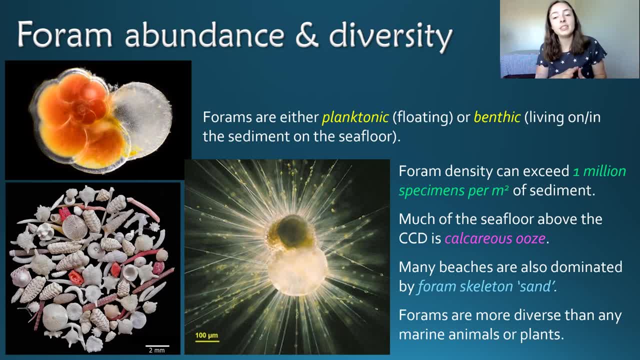 seafloor if they burrow, which they sometimes do just a little bit. but we'll get more into planktonic versus benthic forams when we talk more about their morphology and their ecology. But in terms of abundance and diversity, foram density can exceed 1 million specimens per square. 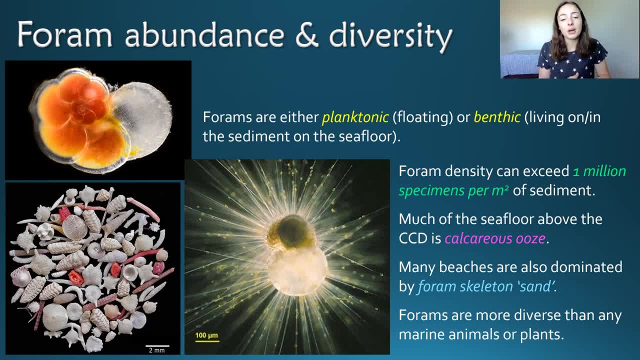 meter of sediment on the seafloor And much of the seafloor above the CCD. because of this abundance of forams not only living on the seafloor but also falling down when they die from the water column is made up of calcareous ooze, which is basically their calcareous 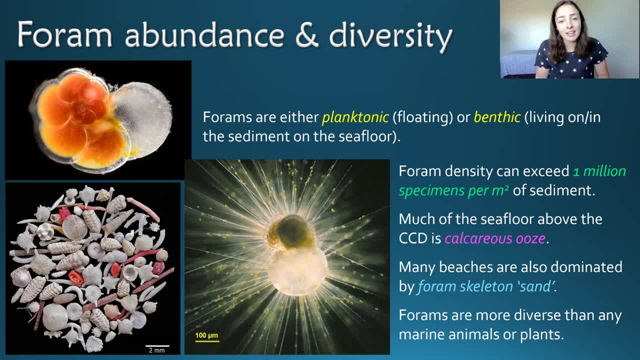 skeletons falling down to the seafloor or dying there and they end up causing this calcareous ooze that ends up making up a lot of that sediment as it gets buried, compacted and preserved, And it's not only seen on the seafloor underneath the water, but even on beaches we can see. 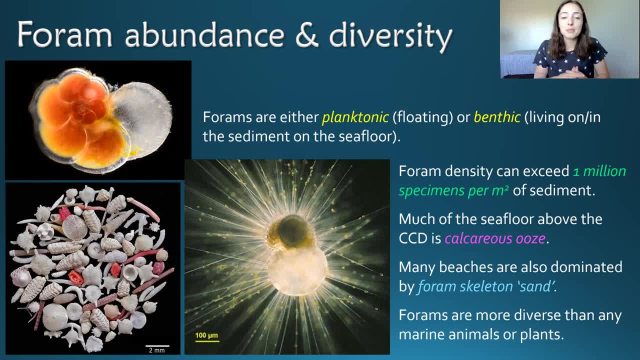 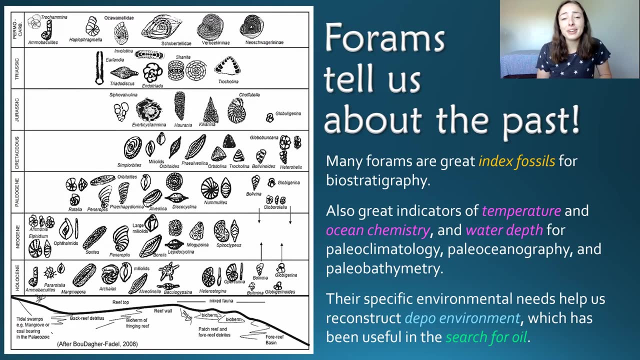 a lot of the skeletons of these organisms, because sometimes beach sand may be completely made up of these foram skeletons And in terms of diversity, forams are more diverse than any other groups of marine animals or plants. But what are forams useful for? Why do we study these things? Well, forams can be great for telling us about the past. 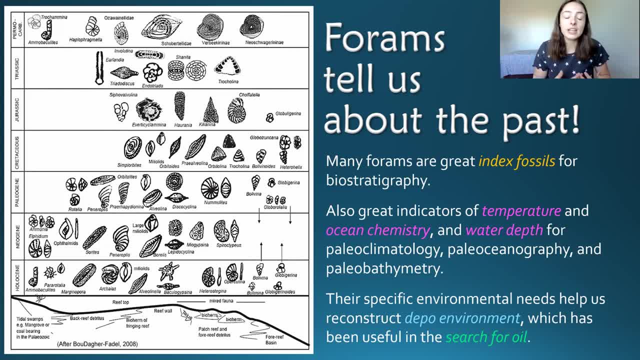 Forams make great index fossils for something called biostratigraphy. If you want to date rocks or figure out the age of sedimentary rocks, it's really hard to do with isotopic dating methods. So if you want to date rocks or figure out the age of sedimentary rocks, 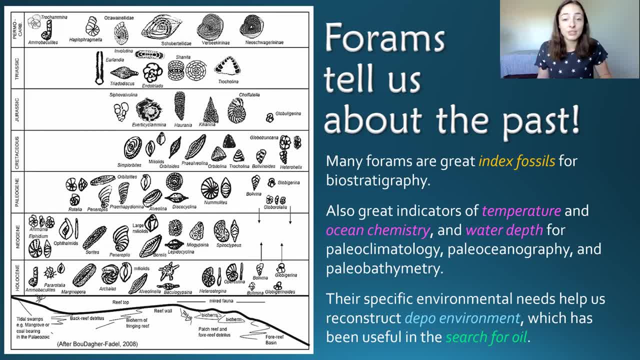 because with sedimentary rocks all the grains have come from different sources and so you're going to get a lot of different ages. But if you have index fossils, you can use them to relatively date those rocks and then correlate those rocks through strata from all over the 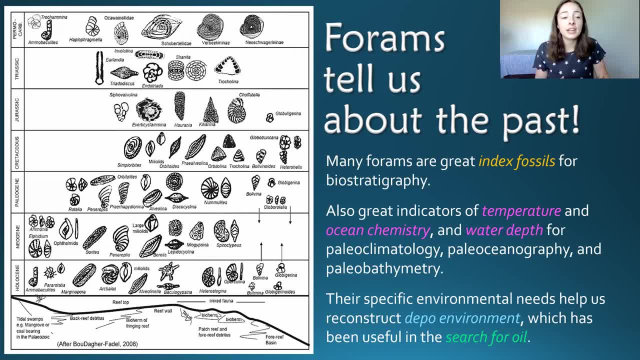 world. But these forams are not only great index fossils for figuring out what time we're at in the geologic timescale when we're looking at rocks, but also figuring out what temperature the ocean was at then, what chemistry was going on in the ocean back then, what depth in the 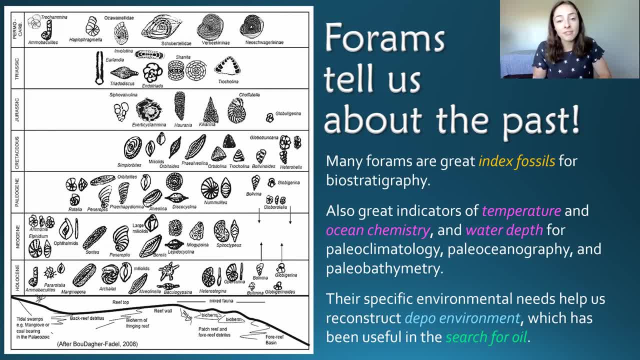 water that sediment was deposited in, because forams have very specific temperature, water chemistry and water depth needs. That means they're very useful for paleoclimate, paleo-oceanography and paleopathymetry respectively, And because of their very specific environmental needs, we can 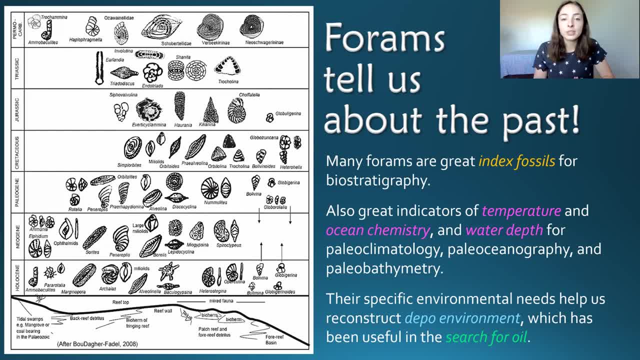 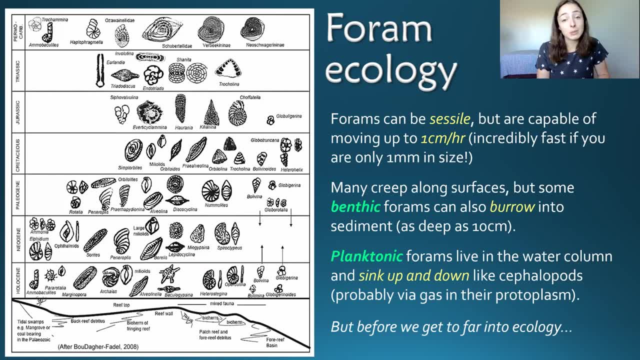 also easily reconstruct depositional environment using our knowledge of what forams are around in those strata, and that has been useful for finding oil. So what are these specific environmental needs that these forams have to deal with? Well, first of all, they're very useful for finding: 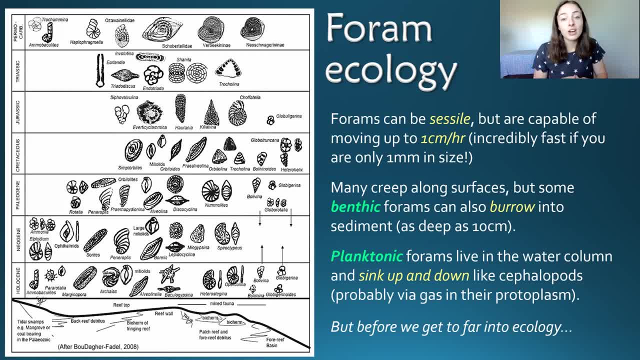 out what time we're at in the geologic timescale when we're looking at rocks. So let's go over a little bit of foram ecology. We're going to talk more about this later in detail, but in general, forams can be sessile or immobile, but they are capable of moving up to one centimeter per hour. 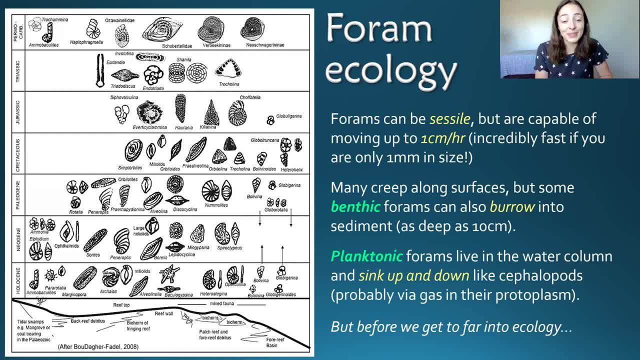 Okay, I know you might be thinking that that sounds really, really slow, but for a one millimeter size organism that's pretty fast. Also, many of them creep along surfaces, but some benthic forams- meaning the ones that live on the seafloor- can burrow into the sediment. 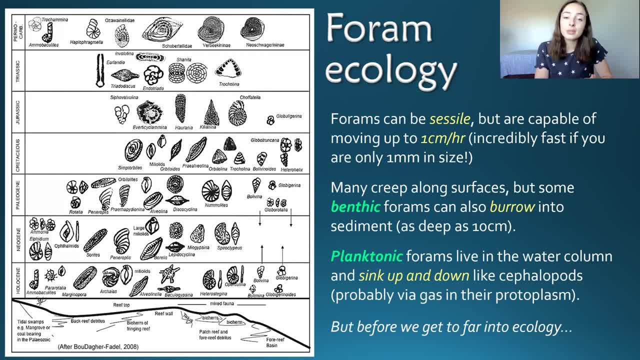 as deep as 10 centimeters. However, planktonic forams- the ones that don't live on the seafloor- live in the water column and kind of sink up and down until they die and fall to the sediment. but the sinking up and down is very similar to cephalopods, which we talked about in the 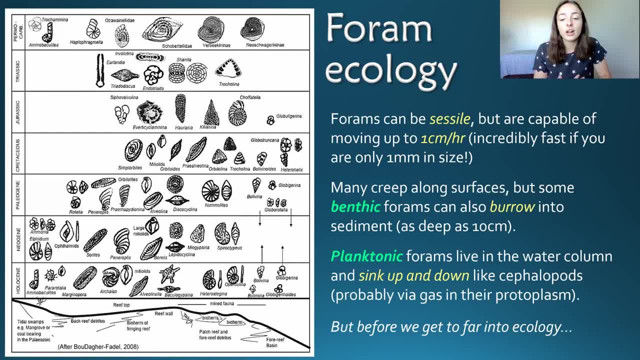 cephalopod video. We talked about how some of them also do that in the water column, and that's because of the way they control gas in their chambers of their shells, and these planktonic forams are similar to that in that they probably sink up and down. 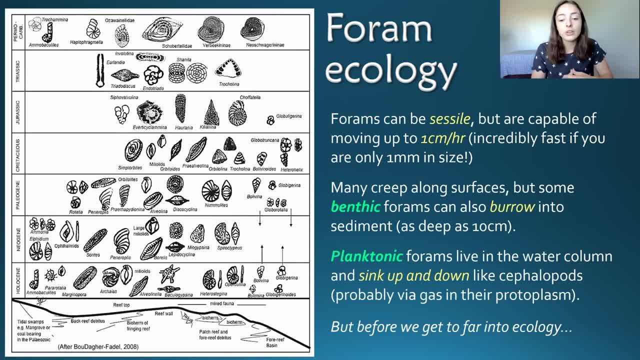 via gas control in their protoplasm or their living material, And I'm going to bring back this figure later and we'll go over it in more detail. So if you're not sure what the heck's going on there, don't worry, we'll talk about that when we get into the more detailed ecology, But before we, 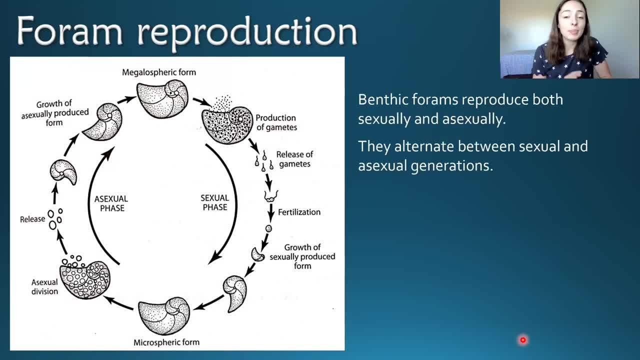 get into that. let's talk a little bit about foram reproduction. Benthic forams reproduce both sexually and asexually. They alternate between sexual and asexual forms as they alternate generations. The asexual or microasexual forams are the ones that reproduce the most. 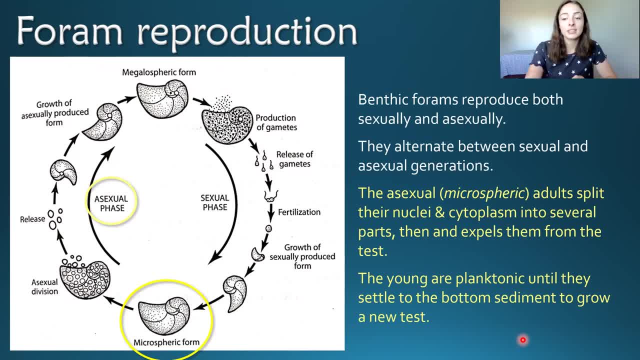 micro-spheric adults split their nuclei and cytoplasm into several parts. then it expels them from their test and the young are planktonic until they settle to the bottom sediment and grow a new test. And so we can see over here this asexual pathway to the sexual adult. But 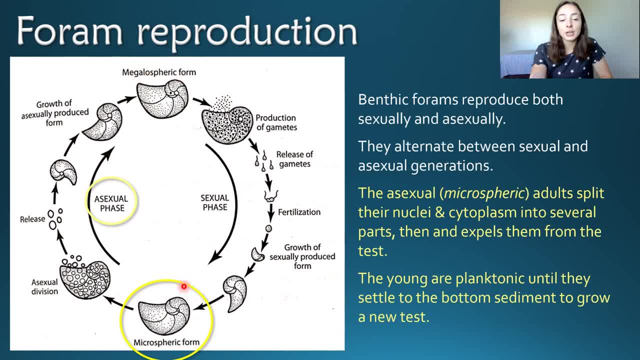 what does this micro-spheric and megalospheric terminology mean? So micro-spheric is a term used to describe the asexual adults in forams, because they have a lot of sex with each other and they have a relatively tiny first sphere which is like their first shell they grow off of. 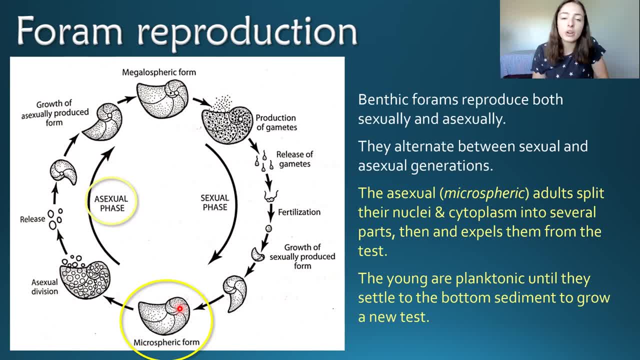 as they grow their test and their chambers. Kind of similar to what we talked about with the cephalopod shells and a lot of different mollusks as well. They have a first part to their shell and then they continue to grow off of that In forams that's typically called the proloculus. 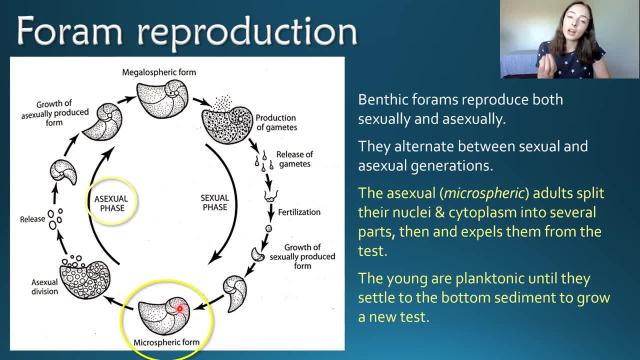 and in mollusks. sometimes we call that the protoconc, but it's this first part of the shell And this sphere is micro in the asexual adults and it's a very large sphere. So it's a very large sphere and it's very large in terms of 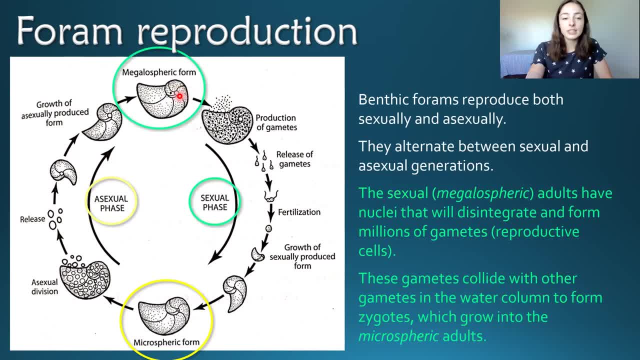 the sexual adult. So it's much larger in the sexual adult And we can see that in the sexual adults or the megalospheric adults, we have the nuclei that will disintegrate and form millions of gametes, reproductive cells, And these gametes will collide in the water column with other gametes. 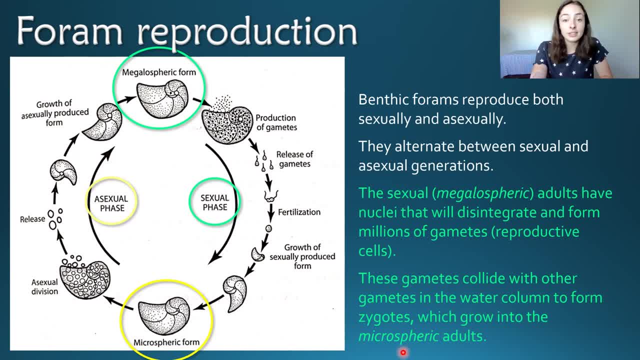 and form zygotes which will grow into the asexual or micro-spheric adults, And so we can see this pathway of sexual reproduction. And then we have the polygamy, which is the polygamy of the asexual adult, And we can also see the polygamy of the asexual adult, which is the polygamy of the. 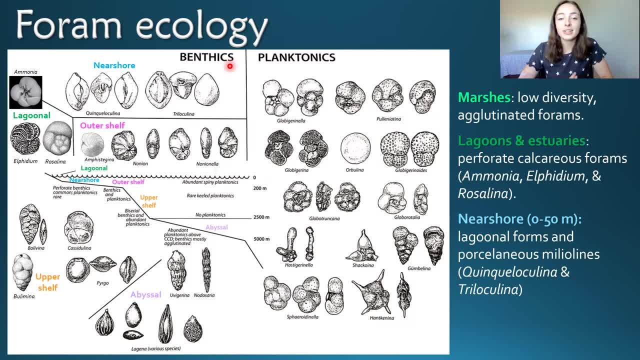 asexual adult. So we can see this pathway of sexual reproduction in this figure as well. So what about the more specific ecology that I said we'd get into? So this is a figure that is just really helpful for remembering which forams live in different environments in shallow marine. 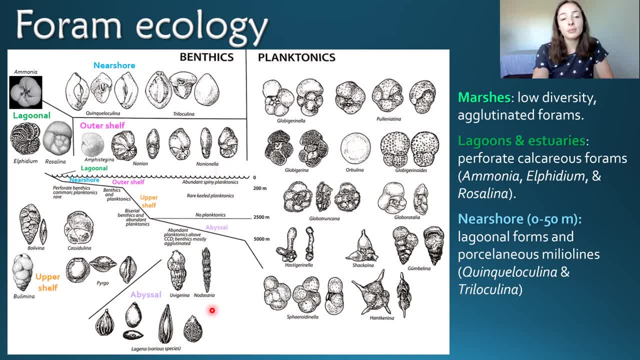 systems. So what we see in this figure is benthic forams on the left side and planktonics on the right side, And then in this little part in the middle we have a marine environment going from lagoonal to near shore, to outer shelf, to upper shelf, to abyssal planktonic, and then you have 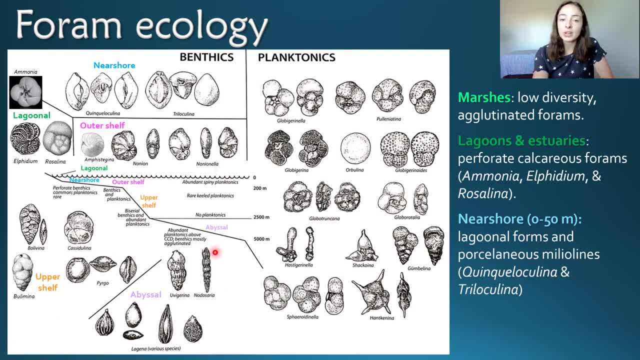 And then in this little part in the middle we have a marine environment going from lagoonal plane and we'll talk about which forams live in each one of these environments. But first we have marshes, which aren't necessarily shown on this figure, but we'll talk about them briefly, Basically, 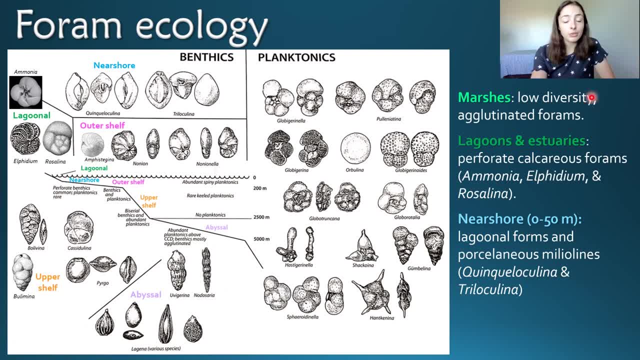 in marshes you will get low diversity agglutinated forams and then, once you get to lagoons and estuaries, as shown here in green, you get perforate, calcareous forams. and we'll talk about different composition of forams when we get to the morphology, but basically perforate just means they have. 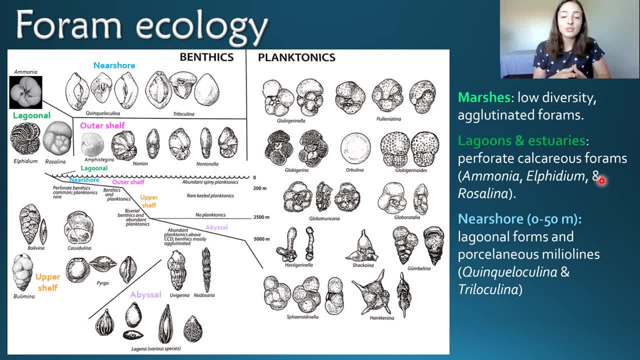 pores in their test, and calcareous just means they're calcite forams, which isn't a common characteristic among all forams and we'll get to that later. So anyway, they're perforate calcareous forams such as the genera ammonia, alfidium and rosalina shown in these lagoonal images over here. 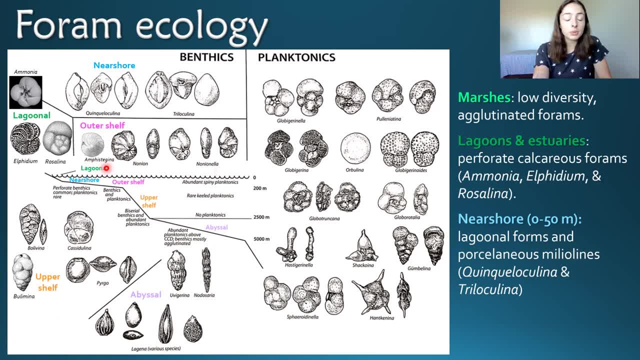 respectively. And then we have nearshore shown in blue here on this environment figure and then up here the forams that are common in the nearshore environment are shown, And these include lagoonal forms, like we just talked about above, but also porcelaneous. 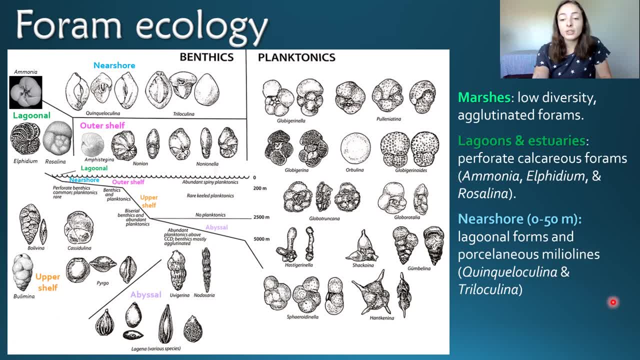 millilines. So millilines are forams that include genera such as crinculocolina up here and trilocolina, and these forms are called porcelaneous because they are made up of smooth calcareous material and look like porcelain In the outer shelf, aka 50 to 200 meters in water depth. we have 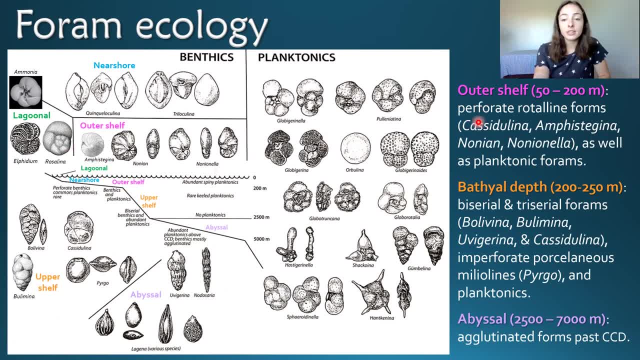 forams shown up here, such as genera casadalina, shown down here in the upper shelf environment, but it's also present in the outer shelf environment. Then we also have amphistagina and that's shown over here in the outer shelf category, And then we have nonian and nonianella. 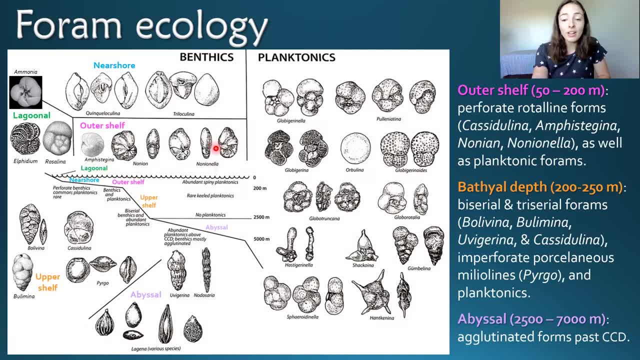 which are both shown over here in the outer shelf category as well, And we also have planktonic forams show up in the water column over here. They aren't typically found, or they're more rare, in the nearshore, in lagoonal and marsh environments, And so they show up in the outer shelf and then 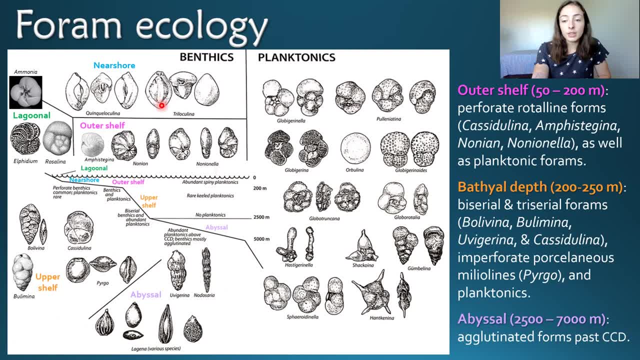 as we'll see, they also show up as we go further offshore. Next, we have bathyldepths, or the upper shelf environment, aka 200 to 250 meters in depth, And we have in this environment benthic biserial and triserial forams, And we'll talk about what biserial and triserial means. You can kind of 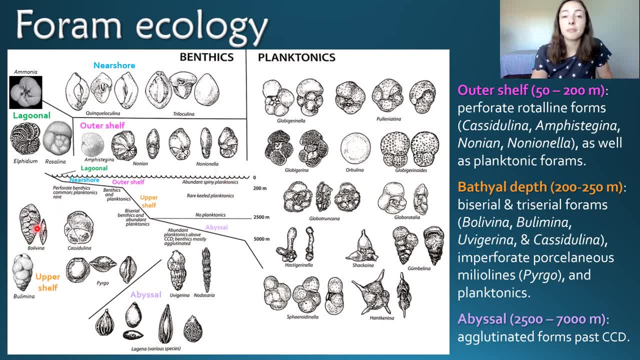 already see it in these forms, like bolivina, which is biserial Aka, it grows a double layer of chambers. And then we have bolivina down here, which grows kind of a triple layer of chambers, And we'll talk about the morphology when we get to test morphology. 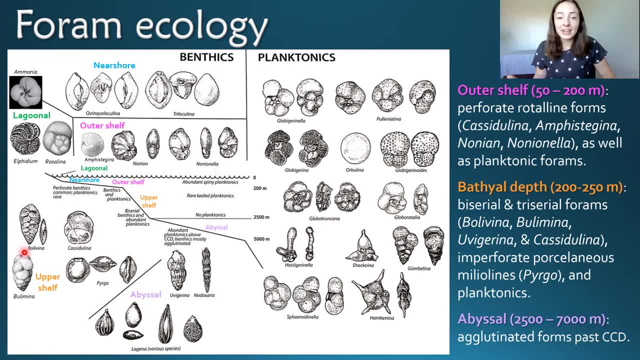 Maybe I should have gone over that first, but we're just gonna go with it. So, anyway, these like to live in this upper shelf environment, as well as uvigurina and casadalina. We talked about casadalina, which also sometimes lives in the outer shelf environment, but uvigurina is shown. 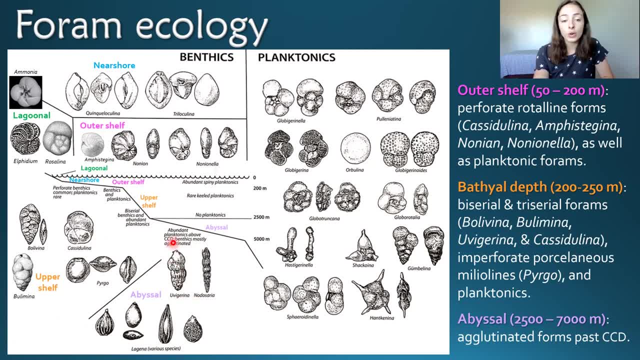 down here We can see that's a uniserial benthic foram, And in the upper shelf there's also imperforate porcellaneous millilines such as the pyrgogenus, And this is shown over here in this spherical-like form with this outer edging around it, And this is similar to the porcellaneous. 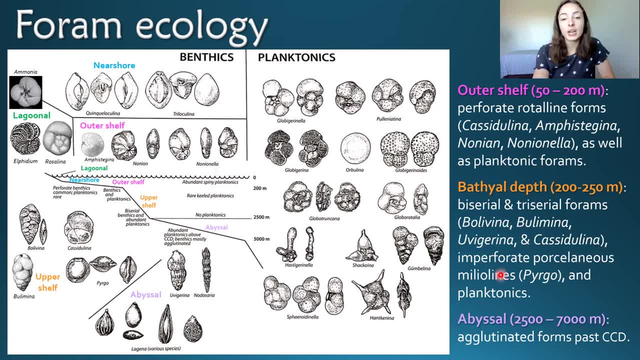 millilines in the near shore environment. but instead of perforate, it is imperforate And obviously it doesn't live in the near shore environment. Then we have planktonics, also abundant in this upper shelf region from 200 to 250 meters. Then we move to the abyssal plane. 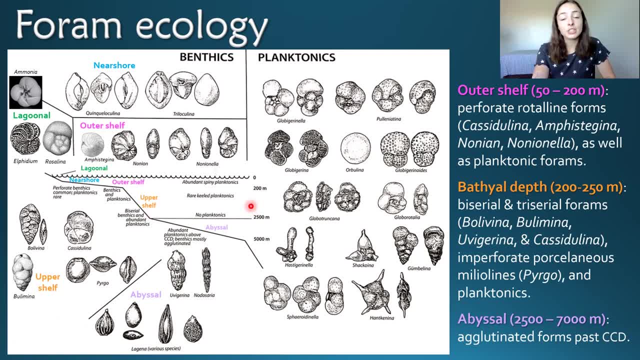 And the abyssal plane above the CCD, which is the carbonate compensation depth, aka carbonate material like calcite and aragonite that many of these planktonic forams build their tests out of, dissolves below this depth and does not above this depth, So above this depth or above the CCD. 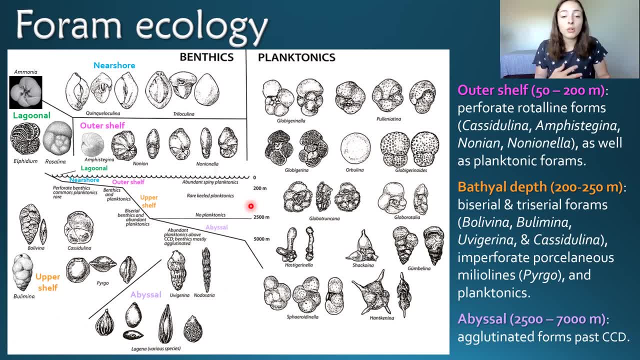 they are present and are abundant in the water column. But as you get below that depth, which is typically around 4,000 to 5,000 meters, you will only see agglutinated forams below that CCD. And that's because agglutinated forams, which we will talk about in two slides, I promise- 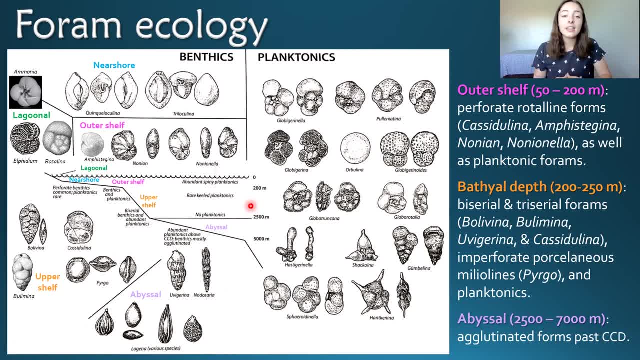 are forams that are not made up of carbonate material. Instead, they are made up of glued together random particles like sand grains or foreign particles at the bottom of the seafloor and dissolved as easily as carbonate material. So agglutinated forams past this depth are common. 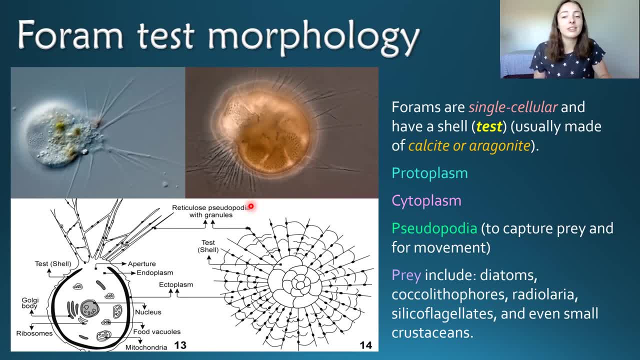 But what about test morphology? I threw out a bunch of terms at you, like agglutinated and protoplasm and test and calcite and all these things, but what's it all mean? So forams are single cellular organisms that have a shell, but we call it a test in terms of four ams, because who knows why it's. 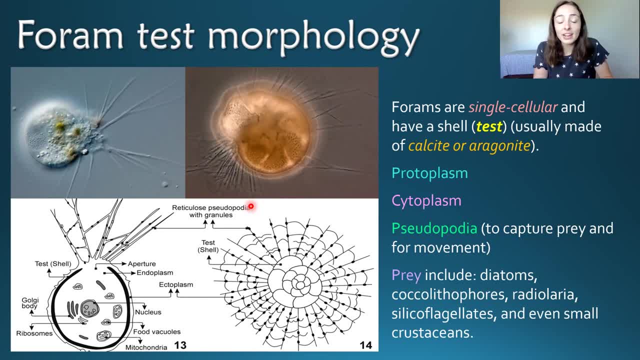 just what we do, and usually it's made up of calcite or aragonite, like we talked about previously, but we only test a few times a week before we are able to get whatever is called a test of everything. The first thing is that we want these flow points to be exogenous to a specific organism. So if you have a 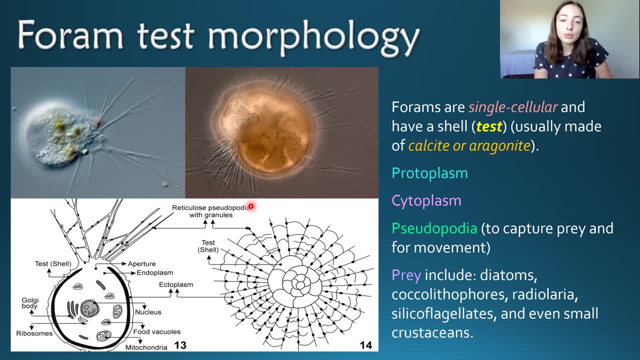 also talked about some forms that aren't, so we'll get to that. and then they also have protoplasm, which is basically their living material in their cell, and then their cytoplasm is, like in any cell, the material that everything else is in, and so their protoplasm encompasses everything in the 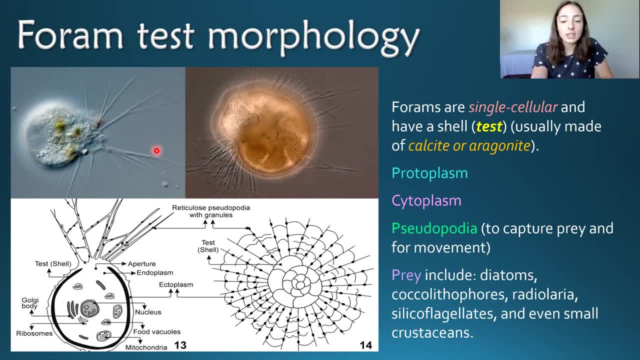 cytoplasm as well as the cytoplasm itself. so that's not very different than any other single cellular organism, or even multicellular organism, for that matter. but in terms of forams specifically, they have pseudopodia, which obviously means fake feet, but they're kind of, in my opinion, somewhat. 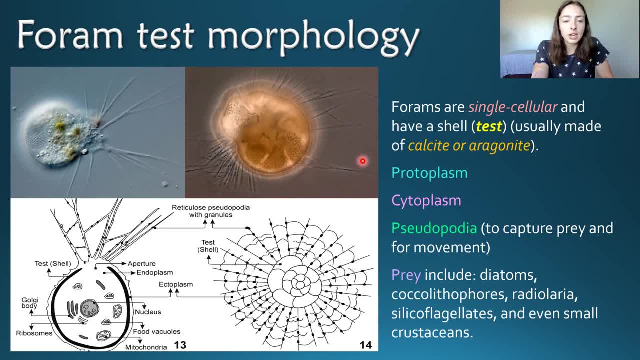 real feet. i mean, these things shoot off the forams, kind of like cilia, and they help them move and capture prey. and their prey that they're catching with these pseudopodia include things like diatoms, coca, lithophores, radiolaria, silica, flagellates and even small crustaceans and, if you're not sure, 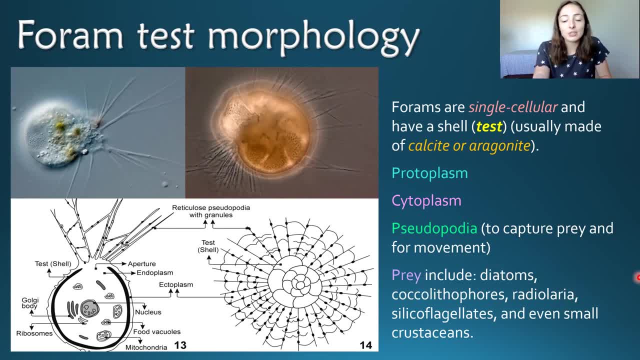 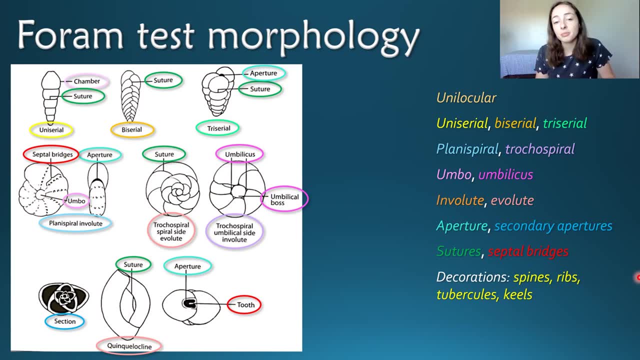 what some of those terms are. we're going to talk about all of these in some upcoming videos, so don't worry. but what about the pseudopodia- other terms i used to describe forams in the ecology slide? uniserial, biserial, triserial, all. 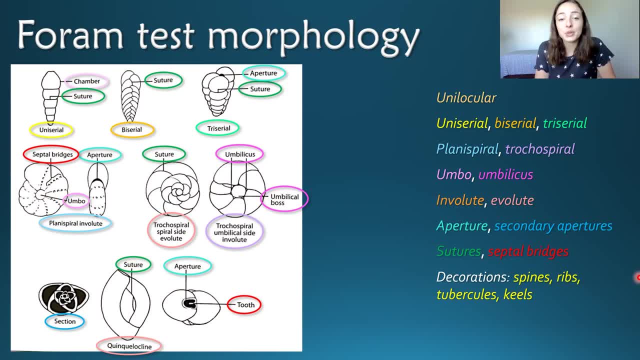 of these things, so let's go over what they mean. sometimes forams can be unilocular, like we saw in the pyrgogenus that lived in the upper shelf environment, and that just means that it has only one chamber. however, that's only common in a few forams, whereas many have multi-chambers. they have: 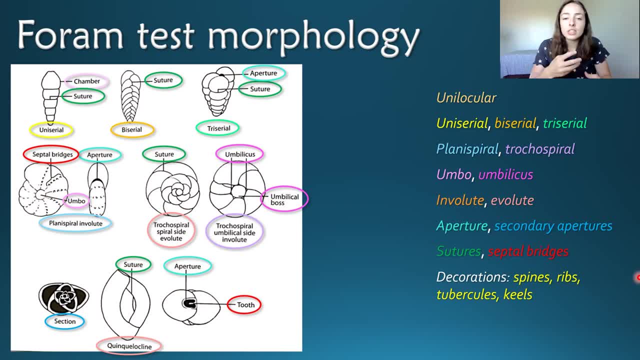 a lot of different chambers, but the way that they grow or add on to the environment is that they grow in a single row and that's what causes so much of the diversity observed in forams. so one way in which forams add on their chambers is in a single row, such as uniserial forams. it's just. 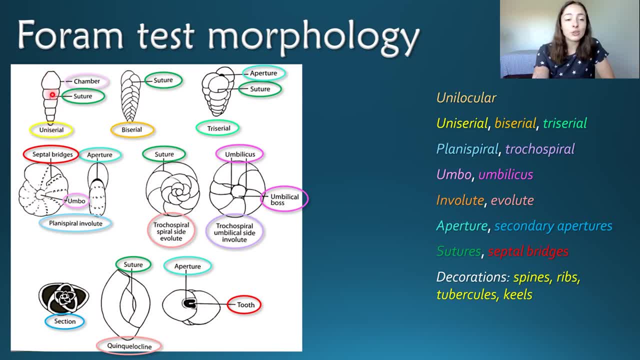 one single like line of added on increasing in size chambers that the foram has. then you can also have biserial, which is two chambers per row that go up in a line similar to the uniserial. then you have triserial, which is three chambers each row. then we have coiled types, kind of like. 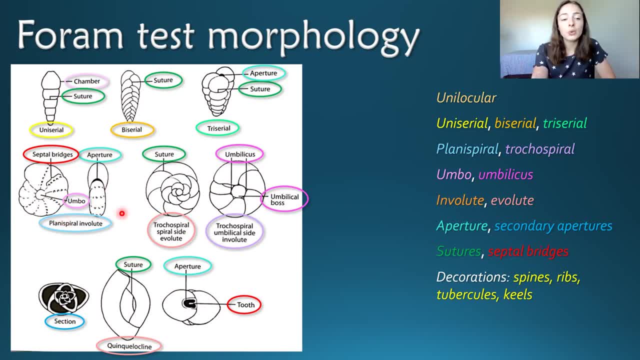 cephalopods, honestly like microcephalopods that can coil in one plane, like planospiral cephalopods, similar to certain ammonites. then you also have trochospiral forms that aren't really shown very well here in this image because we're looking at it from above and below and not from the side. so 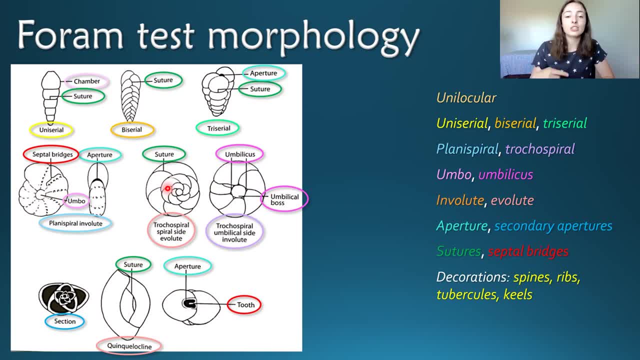 you can't see that the coil is actually not in one single plane. so we're looking at it from the side, so you can't see that the coil is actually in one single plane. it's actually kind of like if you've ever seen a snail shell. the coil goes outward a little bit and this outward coil is 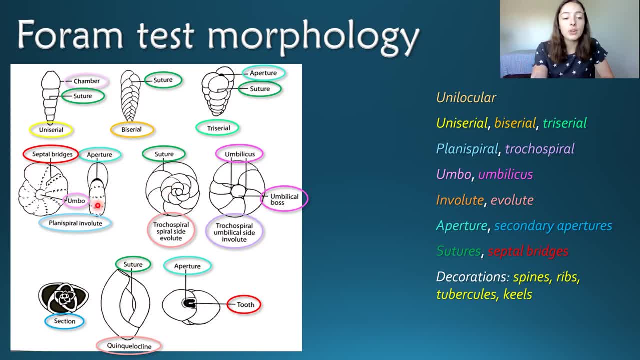 not one single plane, obviously, and therefore not planospiral like the planospiral one we see over here, and it's actually trochospiral and the tippy top of the hat looking spiral is the umbo and the bottom part is the umbiculous. and then we have involute and evolute. here, involute just means 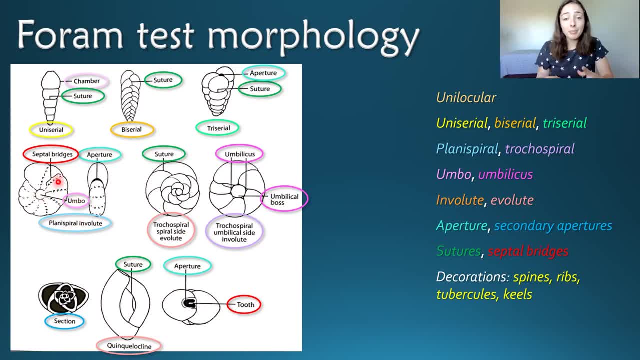 that the chambers of the previous worlds are enveloped or covered up by later worlds, but in terms of evolute, that just means that the inner worlds are not enveloped by the later worlds, and so you can still see the initial worlds and initial chambers that have not been covered up by the later chamber growth things. and then we have the 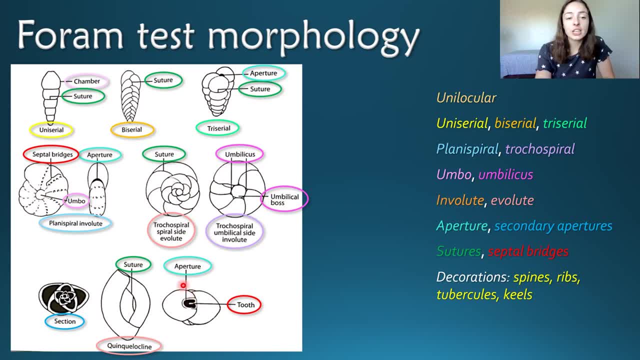 aperture, which is just the opening, that's on the largest chamber or the most recently grown chamber of the foram. and in some forams there are secondary apertures along the other chambers of the test and the lines between the chambers are called sutures, and so we 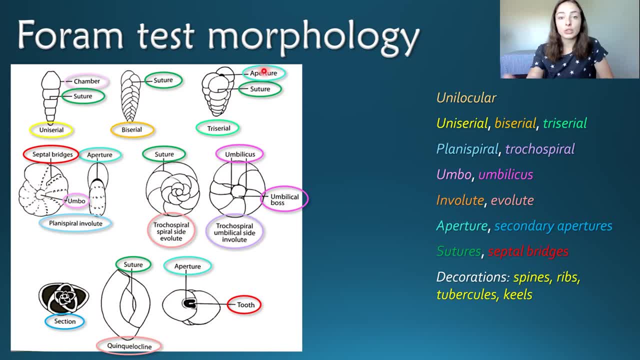 can see these sutures labeled in all of these forums shown here, and sometimes they like to get fancy with their sutures and sometimes they have what's called septal bridges instead because they just wanted to be extra. and then we have more possible decorations down here, like spines, ribs. 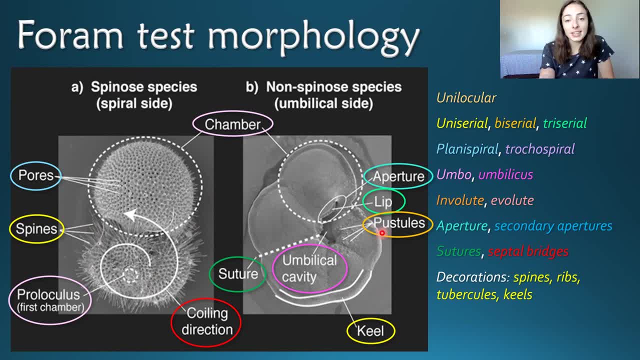 spines shown on this guy over here. then we have this guy over here with no spines and this keel- is this like outer edging part here, which we saw on some of the forms we looked at in the ecology slide? and then they have the other normal things like chambers and sutures between their chambers and 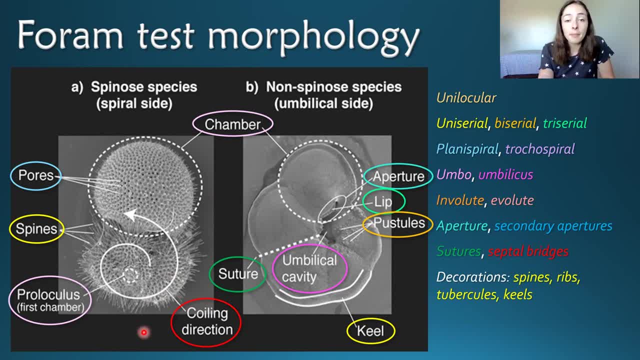 a coil direction which can sometimes tell us a little bit about temperature, and they have an aperture, an aperture lip, an umbilical cavity, the proloculus, the first chamber. they also can have pores in their test and we'll talk more about the test wall structure. 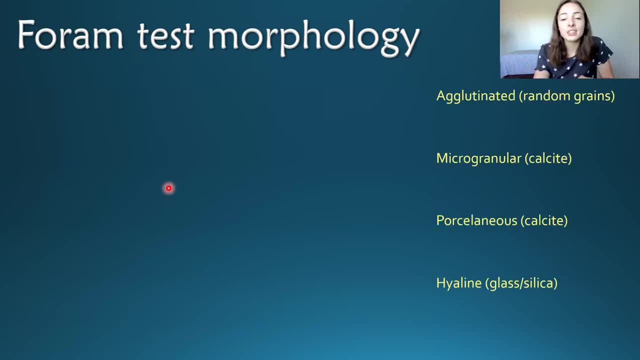 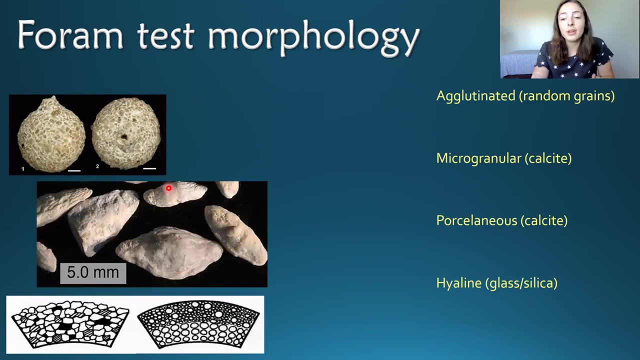 and composition on this slide. so we talked about agglutinated forums and the calcareous forms in the ecology slide, but we also have some other terms on this slide. what are these? well, we have agglutinated forms which are kind of like random grains coming together to make their test. we have 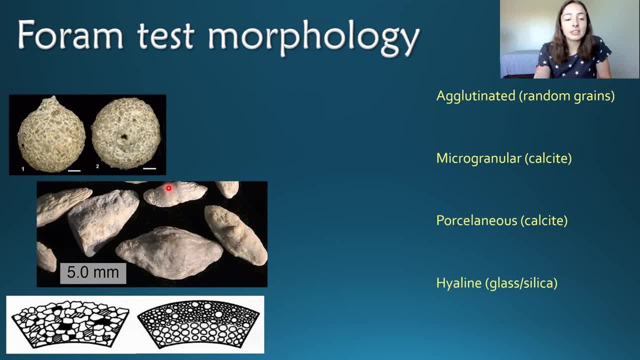 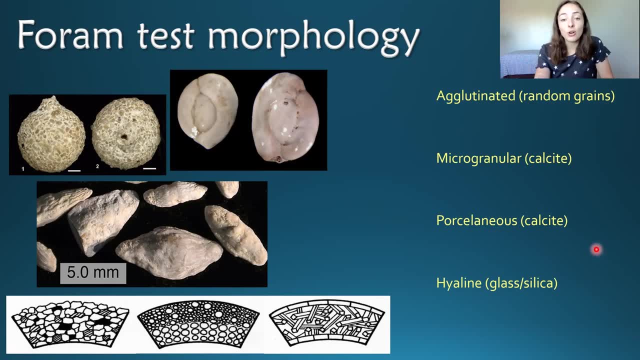 micro, granular, calcitic or calcareous forms like these fusilinids shown here. then we have the porcelain forms, like we saw in the million lines, and we can see that these are also calcite, but they look a lot different than the microcranial forms and that's just because they have a different 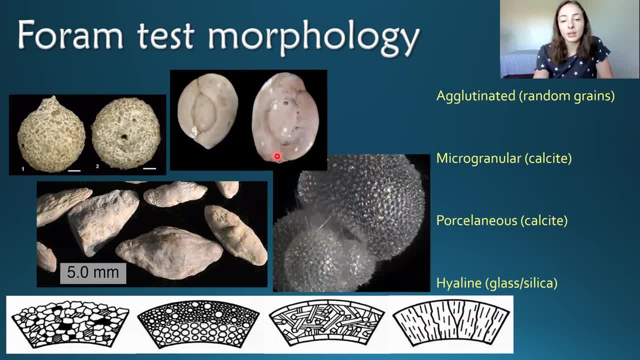 crystal structure of calcite and they come out more smooth and shiny. then we also have high aligned forms, which appear glassy because they're made of silica instead of calcite or random grains. the agglutinated forms, like we talked about earlier, are not typically made with calcite. 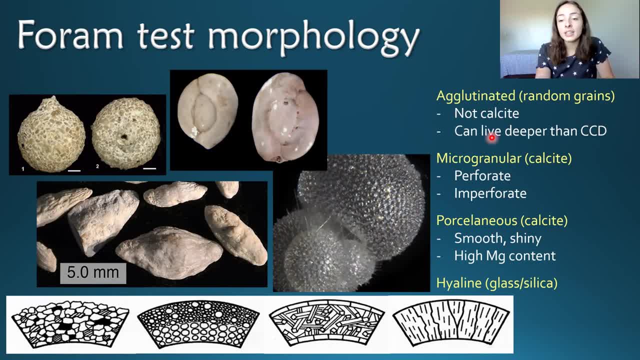 particles- typically they're like sand grains and other foreign particles- and then can live deeper than the ccd because they don't have calcite that will dissolve. they just have random grains that will dissolve and therefore they're fine and can live below that. however, calcitic forms cannot live. 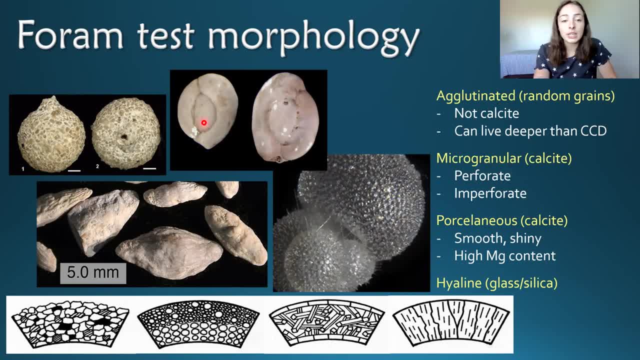 deeper than the ccd and they can be perforated or imperforate, so they can have pores or have no pores. and then the porcelain forms are typically smooth and shiny, like we see here, and have a high magnesium content, which might be the reason that their crystal structure is a bit different, causing 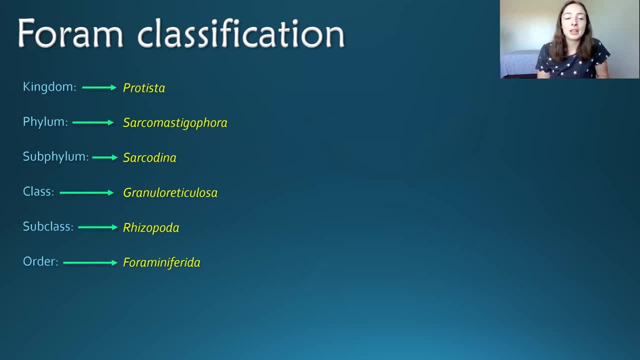 them to look porcelainious rather than micro granular. so what about 4m classification? we already talked about how they are protists and they're in this phylum, sub phylum, class, subclass and order listed here. that I don't want to repeat because they are very hard words, but in terms of 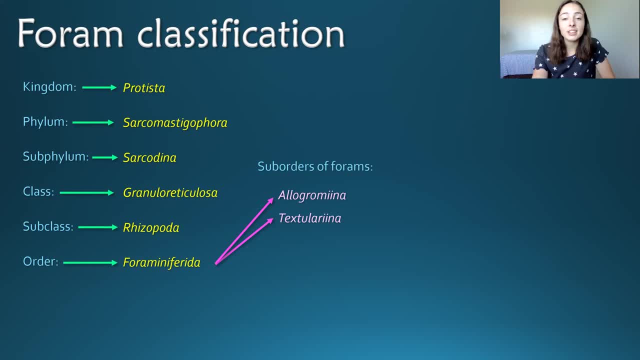 sub orders of forums. these include alogamina, textularina, laganina or laganina, fusilinina or fusilinina, millilina, rhodolina or rhodolina, and clobigerina, and the first one is characterized by single chambered or unilocular tubular round or flask shaped. 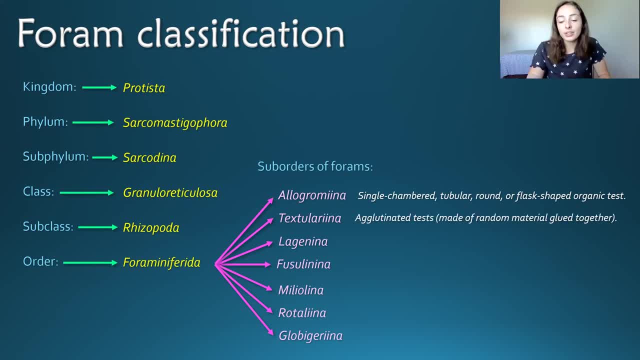 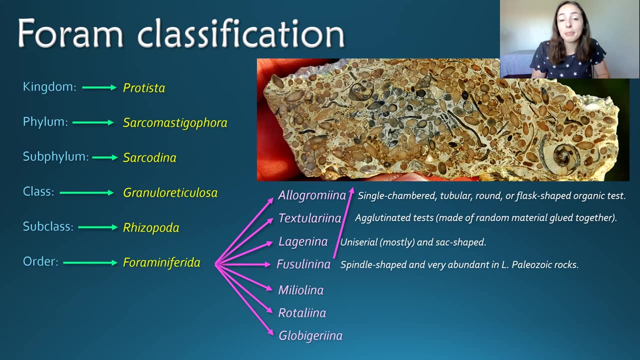 with organic tests. the second includes agglutinated forms, the third is typically uniserial and sack shaped. and the fourth, or the fusilinids, which we'll talk about more in the next slide, are spindle shaped and very abundant in the late Paleozoic, and this abundance in the late Paleozoic as well. 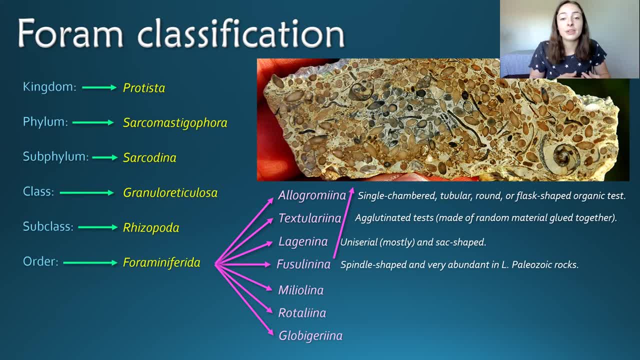 as their very specific morphology and their geographic widespreadness makes them really good index fossils. but we'll talk about those in the next slide. then the millilines are porcelaneous tests. we saw those in the ecology as well as the previous slide when we talked about different compositions of 4m tests and their shiny calcareous tests that. 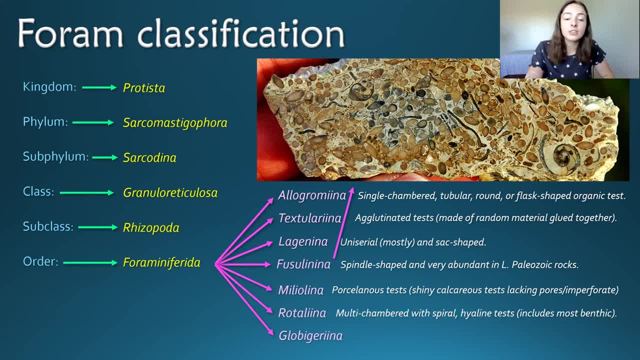 typically lack pores, aka imperforate, and rhodolina includes multi-chambered forms with spiral or Highline tests, so like glassy tests, that includes mostly benthic forums, and then glabrides are planktonic, not been thick and they have bubble-like Chambers that are arranged in expanding spiral and 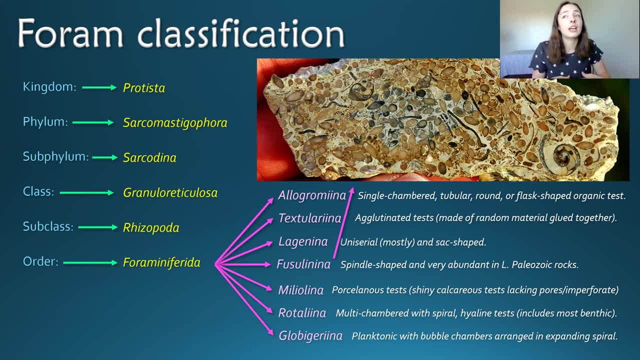 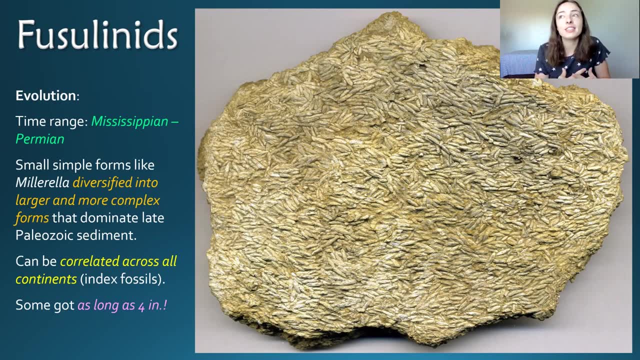 because they're typically easier to remember, because clavigerine sounds kind of like globular and they look globular because they're bubbly. but now I want to talk a little bit about fusilinids, because these are really important index fossils and I don't know about you guys, but my professor 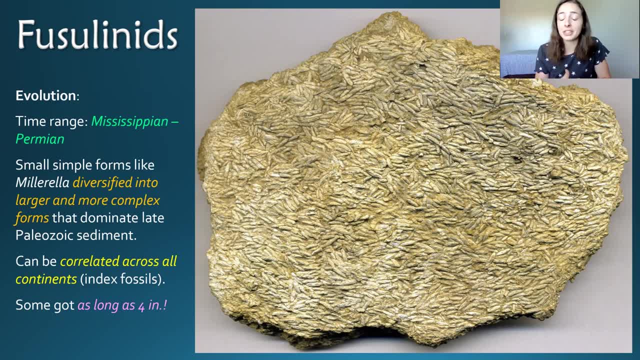 really liked to focus on these, probably because he studied them for a lot of his life and he was really an expert in them. but anyway, these guys are like little rice-grained football shaped little things, and I'll show more cross sections of them here in a second so you can see they're. 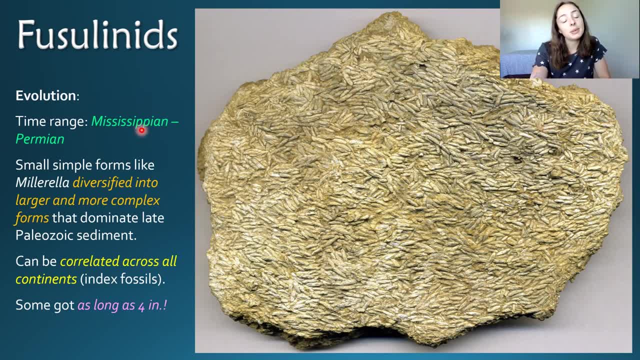 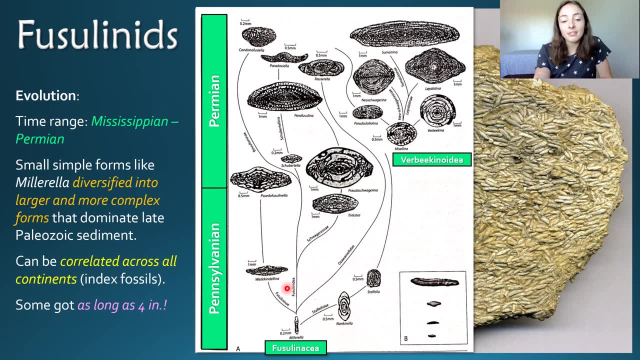 an internal complex structure. but these guys lived from the Mississippian to the Permian and in terms of their evolution, they evolved from small, simple forms like millerella- this tiny form down here that was relatively simple and internal structure- to much larger and complex forms in the late. 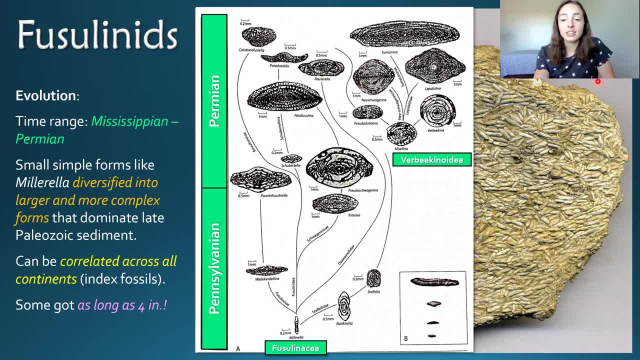 Pennsylvania and Permian periods of the late Paleozoic, and this widespread domination of these forums led to them being able to be correlated across all continents, making them like index fossils. and another thing I think is just cool is that they got as long as four inches. 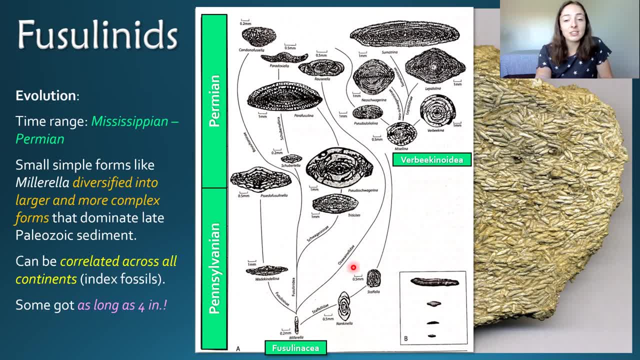 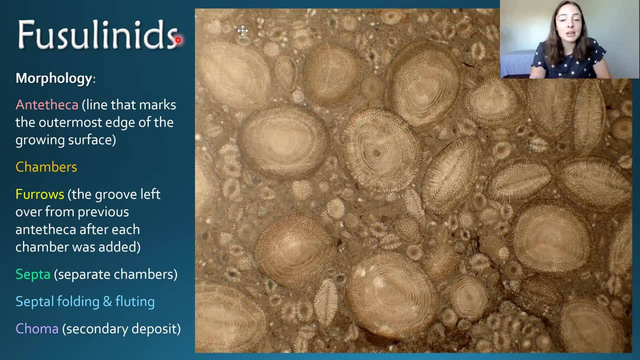 you can see, from this size around 0.2 millimeters to four inches. that was an incredible evolution and really really crazy for something that's single cellular guys, but in terms of their morphology, which can be really important if you are maybe taking a test on forums and your 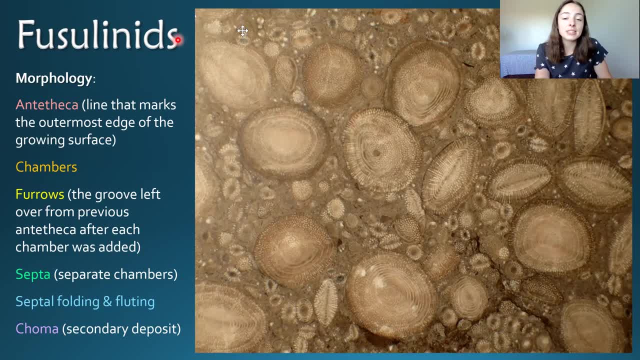 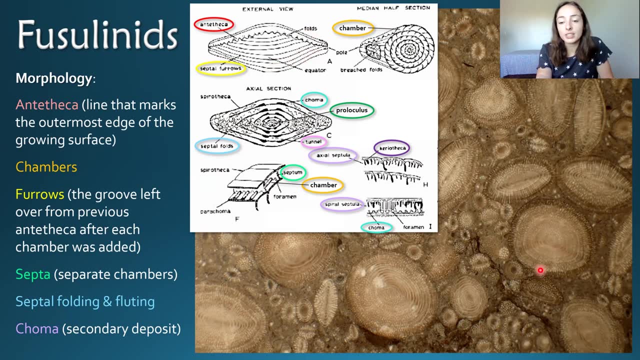 professor likes fusilinids. I'm gonna go over some of the terms that go along with fusilinid morphology. what we can see here is their football shape, and we can see this also in this rock slab that's in the background. here they have a football-like shape in their axial section or their axial cut. 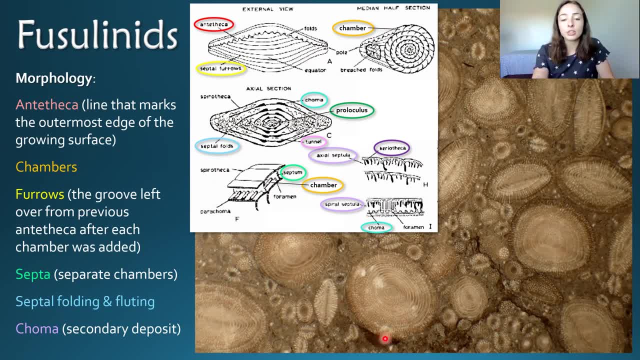 along the long ways of their body and then they have a rounder shape. if you cut them in the equatorial section, so along their like equator, or this like cut right here, that you would do. if you cut that it would be circled. if you cut along this way, it would be a football shape and that's what 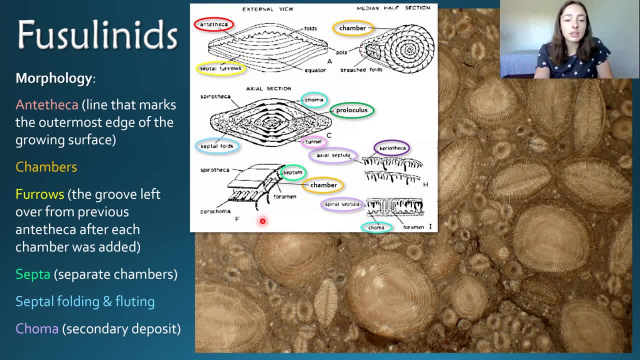 we're seeing in this rock slab, and so we look at some of the labels here we can see some similarities with the overall general form: morphological terms like proloculus, their first chamber, which can be relatively tiny or relatively large depending on whether they're microspheric or megalospheric at the time, aka an asexual adult or 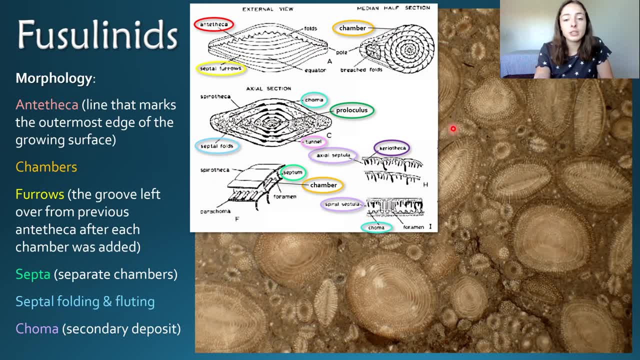 a sexual adult respectively. we also see some other terms listed here that are also labeled. we have the antithyca, which is the line that marks the outermost edge of the growing surface shown here. it's kind of ripply and these are just folds, and sometimes these folds can cause an overall 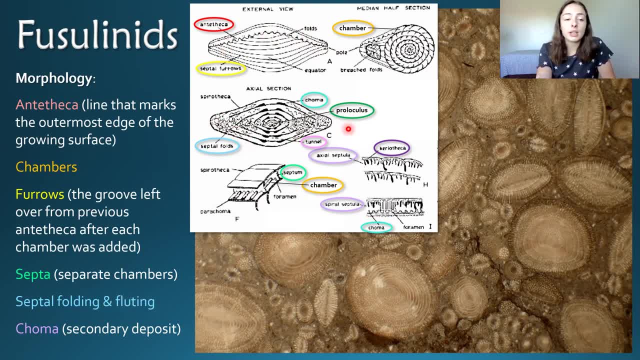 structure typically termed fluting or septal fluting. and then we also see chambers. that's another common characteristic among all forms we've already talked about- and so these are obviously multi-chambered, but they're not uniserial or bi-serial or any of those morphologies. they're 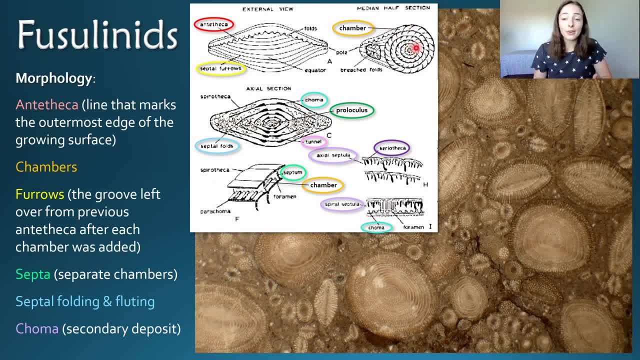 actually coiled and they are technically plan a spiral. but instead of coiling in one plane and then just being like a thin coil thing, they're plan a spiral. but they're also called fusiform in their morphology because they have this elongated planet spiral form. 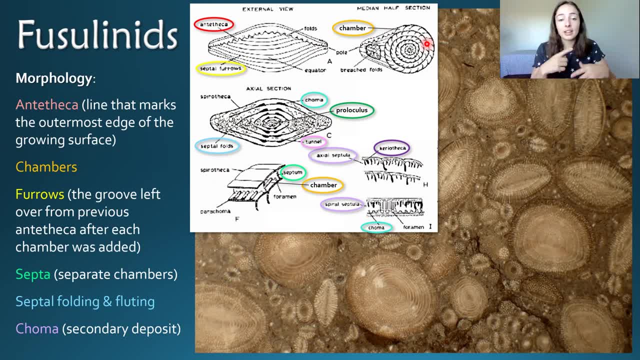 that kind of you know goes out in this football shape as they spiral around their proloculus, and as they spiral they add a chamber at a time, moving their antithyca one chamber forward. each time it adds a chamber, and each time it does so this causes burrows to form, aka the grooves left over. 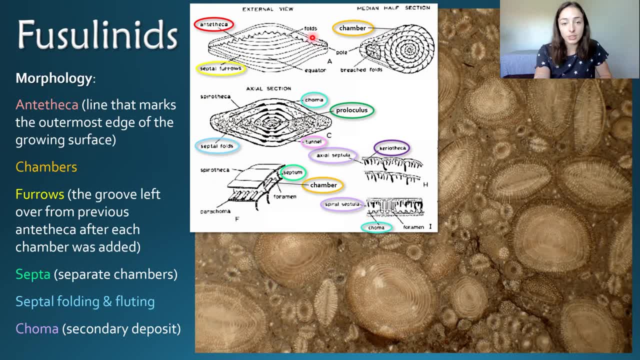 from the previous antithyca after each chamber was added. so these burrows can be seen in these lines here in the outer part of the forearm, and if you cut the internal part you can't see the furrows. it's just on the outer part that you see the furrows, and then the septa are. 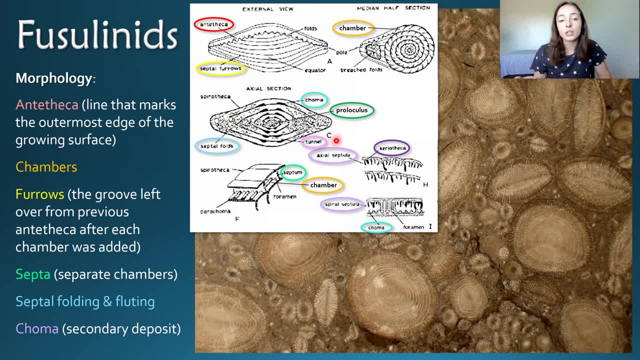 what separate each chamber. so, similar to what we talked about earlier with sutures, it's just that the septa separate each chamber, and so we can see these septa are shown here. after each chamber there's this little tick. those are septa. we can see the axial septula shown here. septula are just. 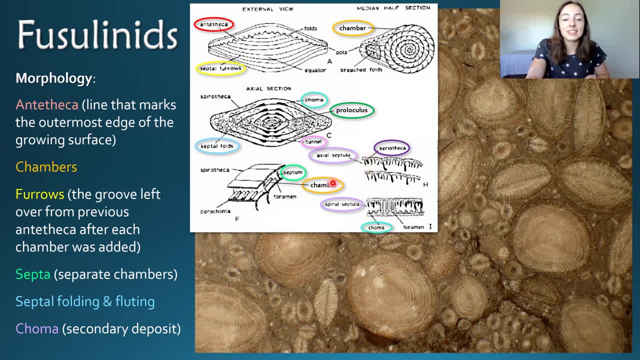 septa that don't reach all the way to the bottom, um, whereas the septa are the complete separations of each chamber that do reach to the bottom and do separate each chamber, we also have something called coma, which are kind of secondary deposits or these dark, lumpy things shown here and as you 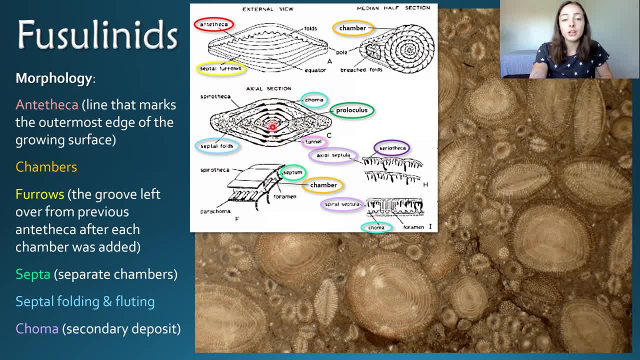 can see, there's this like x looking shape of coma shown in the axial section, and this x shape of coma surrounds something called the tunnel. this part in the middle of the septa is called the tunnel that doesn't have any secondary deposits or doesn't have any coma, or comata plural, that is. 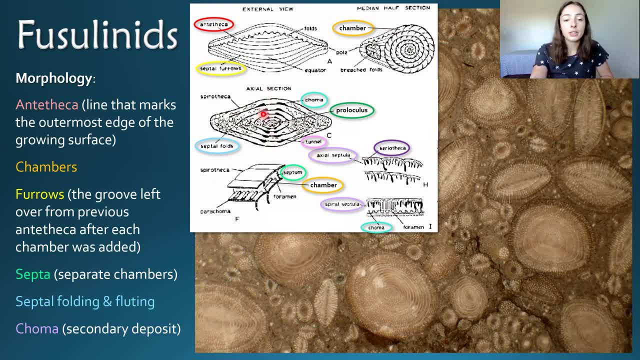 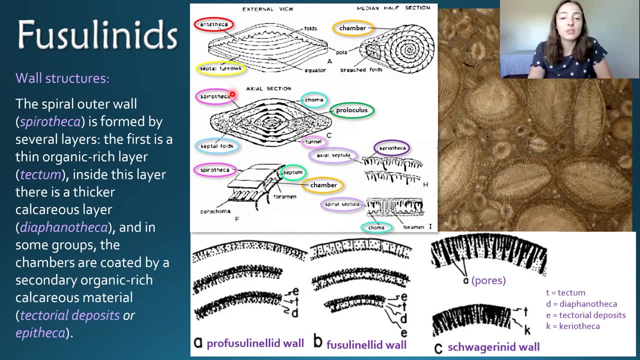 called the tunnel, that inner part there, that lighter part, and then the x surrounding it is the comata or coma singular, and we also have some terms over here like karyotheca, or over here like spirotheca. well, we'll talk about that as we get into the wall structures, wall structures of fusil. 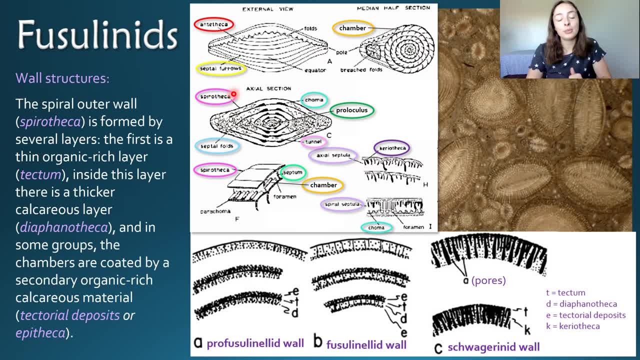 linens can get a little complex and i had to draw these so many times for my periodology class. i'm going to go into them now. basically, the spirotheca is the spiral outer wall, which actually is formed in several layers, and we'll talk about what these layers are in just a second. 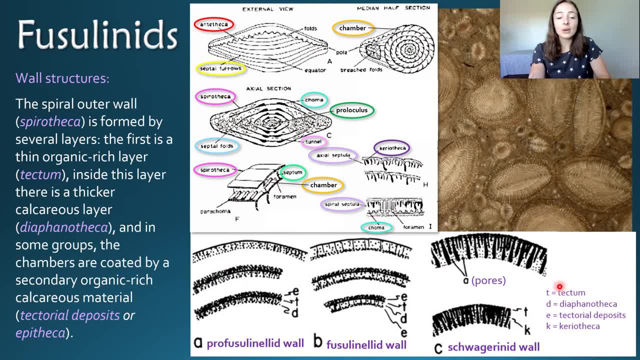 first i got to tell you what's going on down here. what does it all mean? now, what these three different structures represent is kind of the evolutionary trend of fusilin it's. first they had profusilinellid wall structures, a very ancestral, simple wall structure shown in a. then we had b. 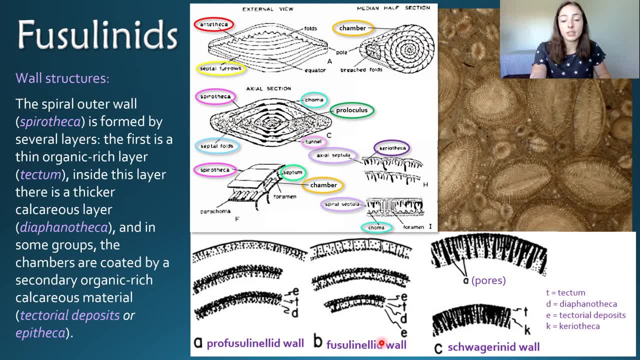 with the fusilinella wall structure, still fairly simple, but there's an extra layer we'll talk about. then we have c, the schwagerin wall structure, and these were a little bit more simple, in some ways a little bit more complex than others. so we'll talk about all three of these wall structures basically. 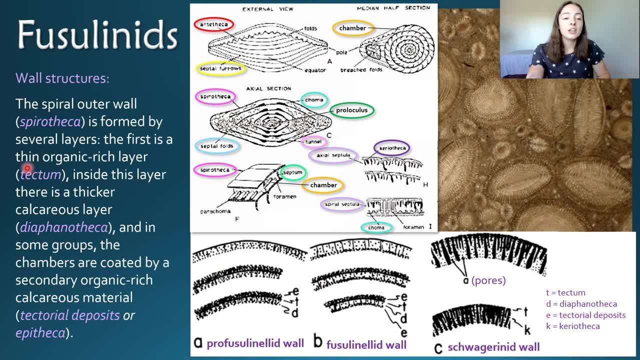 these several layers that make up the wall structures include the tectum, which is the first organic rich layer, this dark line labeled t and that's also labeled in the fusilinellid wall structure and the schwagerin wall structure. and those are just the first organic rich layer, the tectum, and then inside this layer there's a thick 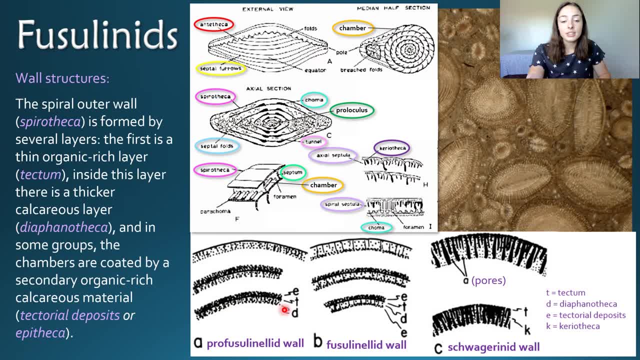 calcareous layer or the diaphanotheca. this is relatively thick, so we can see that's much thicker than the tectum layer. that diaphanotheca is calcareous instead of organic and that's shown in both of the first two wall structures, the profusilinellid and the fusilinellid wall structures. 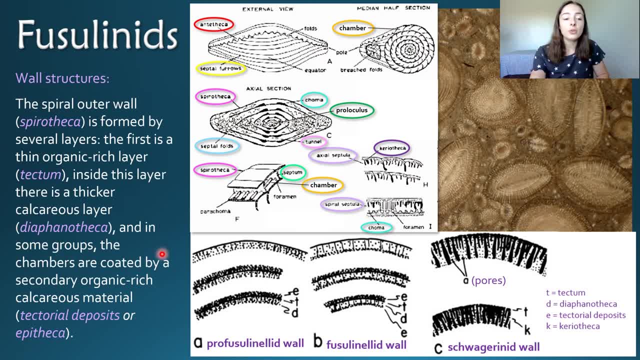 and also in both of these wall structures you have the chambers coated by a secondary organic, rich calcareous material, so organic and calcareous material, and the tectorial deposits labeled by e, also sometimes called the epitheca, and this e label is shown up here in the profusilinellid wall. 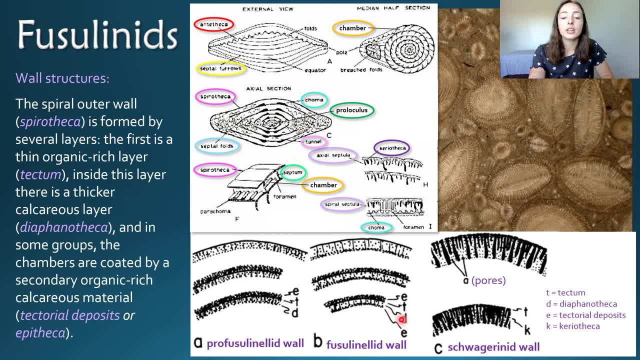 structure and both above and below the wall structure. in the fusilinellid wall structure that was kind of the trend in evolution from the profusilinellid to the fusilinellid- was the addition of an additional secondary tectorial deposit or epitheca below the wall structure. 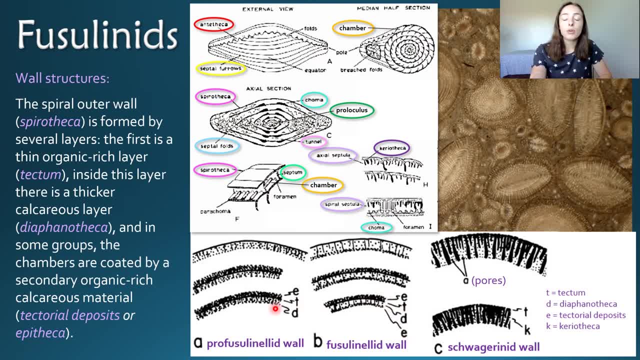 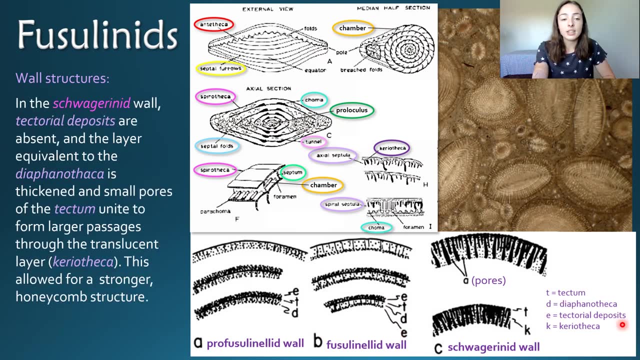 and so this tends to be a four layer structure and the profusilinellid tends to be a three layer structure. however, as we get over to the shragaranid wall structure, we see that there are only two labels, and they're lacking the diaphanotheca as well as the epitheca, or tectorial deposits. 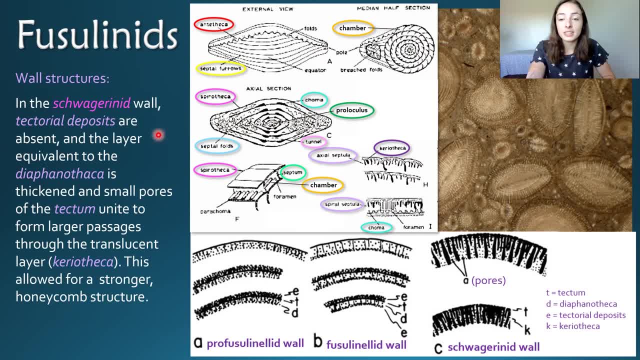 so, in terms of this wall structure, we have tectorial deposits absent. we also have a layer equivalent to the diaphanotheca that is thickened and small pores of the tectum unite to form large passages through the translucent layer and that is now called the karyotheca. this karyotheca, 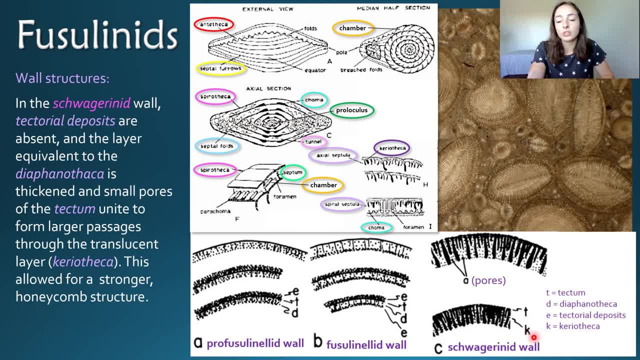 structure is this complex, now honeycomb structure that allows the shragaranid wall structure to be stronger. this is what we saw up here. this was the karyotheca of this shragaranid wall structure shown here as well as down here, and they also have pores labeled here and this wall structure. 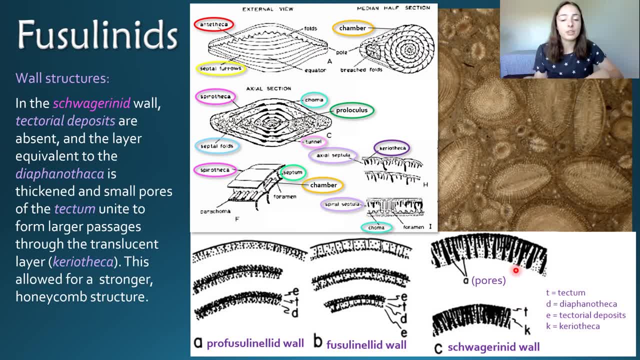 was stronger. so the evolutionary trend from profusilinellid to fusilinellid to shragaranid was going from relatively weaker to much stronger in their structure. so if that's the evolutionary trend for fusilinellids, that's great rachel. but what are the evolutionary trends among forams as? 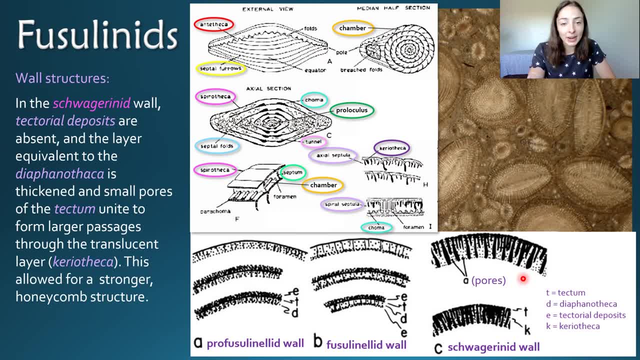 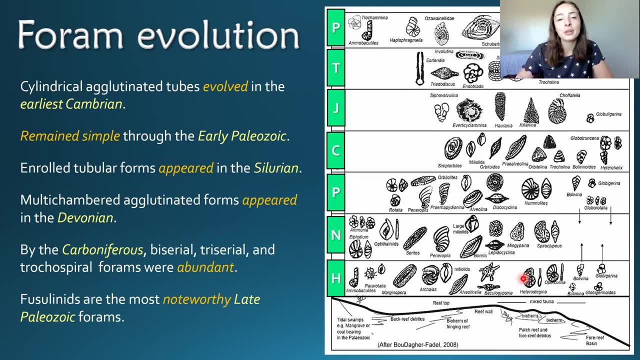 a whole. we're here to learn about forams, not just fusilinellids, right? okay? yeah, you're right. so let's move on to foram evolution as a whole. first, in the earliest of the camprian period, we see cylindrical agglutinated tube forams evolve, and then the foram evolution. 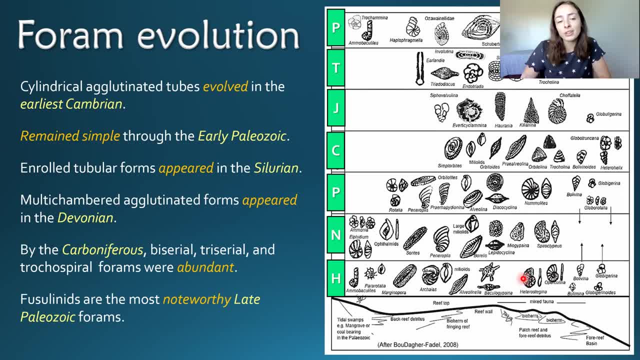 was a little bit boring throughout the early paleozoic, in which their morphologies remained relatively simple and then enrolled tubular forms appeared in the solarian and then we had multi-chambered agglutinated forms appear in the devonian and then by the carboniferous, which is 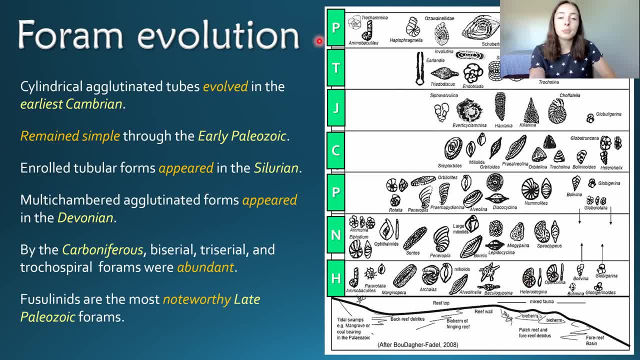 where this figure starts. this figure over here shows from the pennsylvanian permian time to the triassic, jurassic, cretaceous, paleocene, eugene and holocene, so from older to younger going down, and also shows ecology of the forum, going from near shore to offshore, left to right, and by the carboniferous we see biserial tricerial. 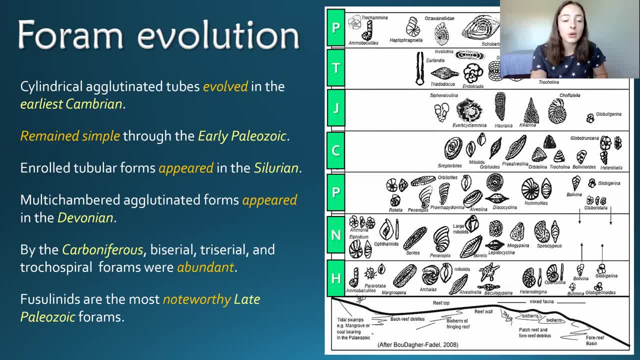 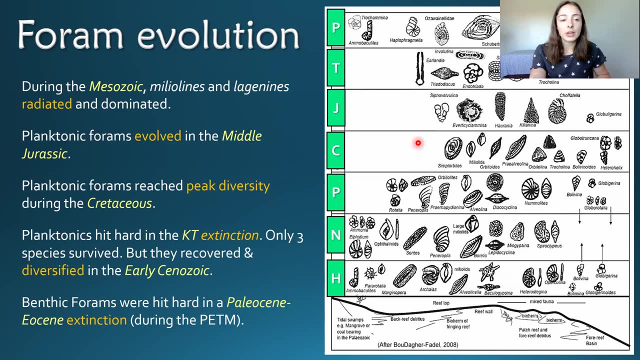 and trochospiral forms as we see up here in the pennsylvanian permian row. then we also note down here again: fusilinids were probably the most noteworthy late paleozoic forams just because of their really useful index fossil use, and so we see these up here as well. but during the mesozoic 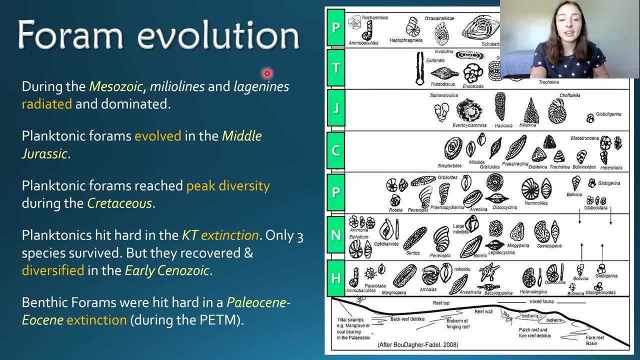 after fusilinids had died, million lines and laganines or laganinies, were allowed to radiate and dominate during this time. and then planktonic forums actually first evolved in the middle jurassic. they weren't even around in the entire paleozoic. it was from the cambrian to the jurassic. 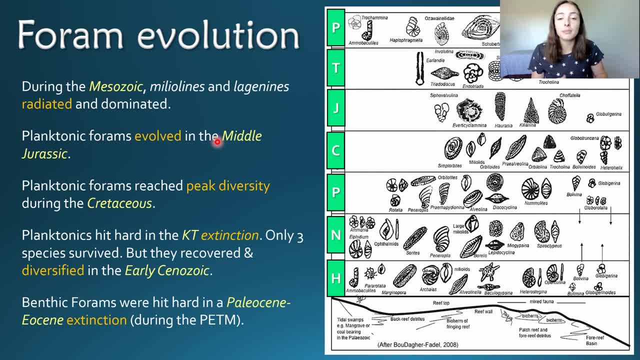 the benthic forums were the only things around. then planktonic forms evolved in the middle jurassic and then you had planktonic forms hit their peak diversity really soon after that in the cretaceous. and then planktonic forms were hit really hard in the kt extinction only three. 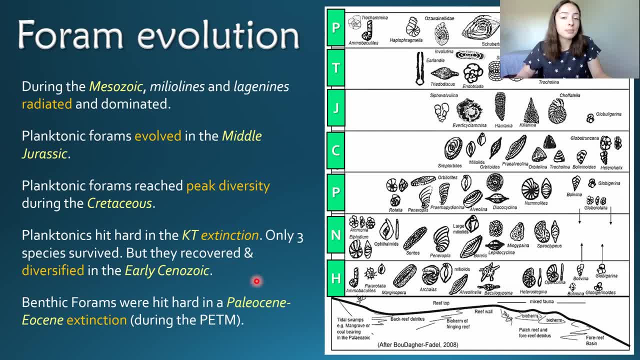 to recover and diversify in the early cenozoic, and now all of the planktonic forums that we see today have evolved from those initial three species that survived the kt extinction. and then the benthic forums were hit hard in the paleocene eocene extinction event during the petm, which 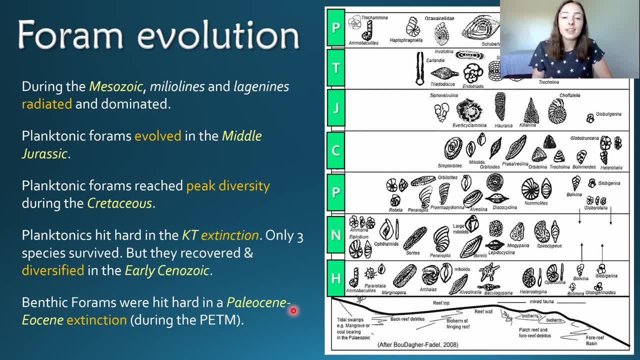 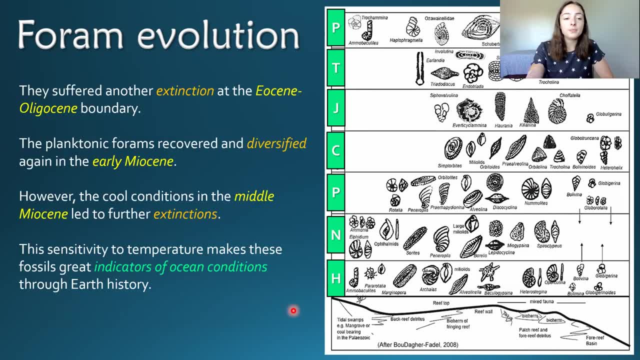 is the paleocene eocene thermal maximum, a very warm period that likely melted methane hydrates, altering the bottom water composition of the ocean heavily enough to kill a lot of these forums. and then they suffered another extinction event at the east scene, a legacy boundary where things started to cool off because nothing likes rapid change, whether it be warming or cooling. 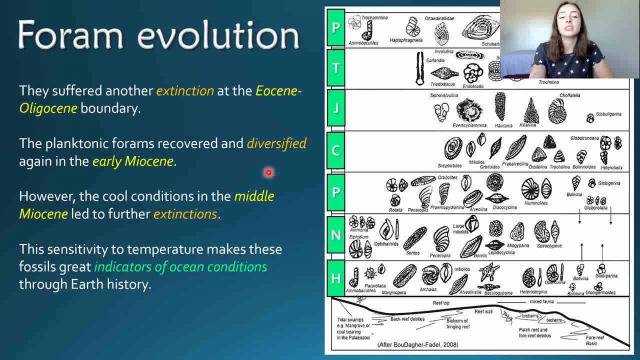 and then, after this extinction event, you had planktonic forums recover and diversify in the early miocene, when things began to warm up again, but then the cool conditions in the middle my scene led to further extinctions and this remarkable dying and recovering and sensitivity to temperature. 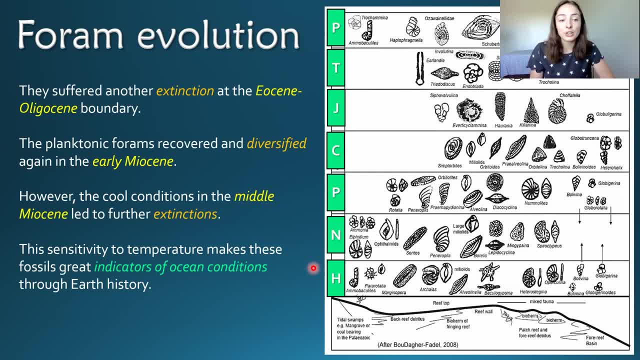 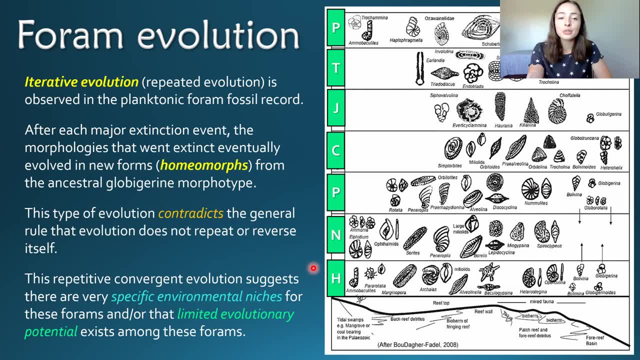 makes these fossils great paleo thermometers or indicators of ancient ocean conditions throughout earth's history, like we talked about previously, and in terms of evolutionary trends, some are really, really cool trends we're seeing, especially in planktonic forums. for example, we see iterative evolution or repeated evolution, observed in planktonic forums throughout the 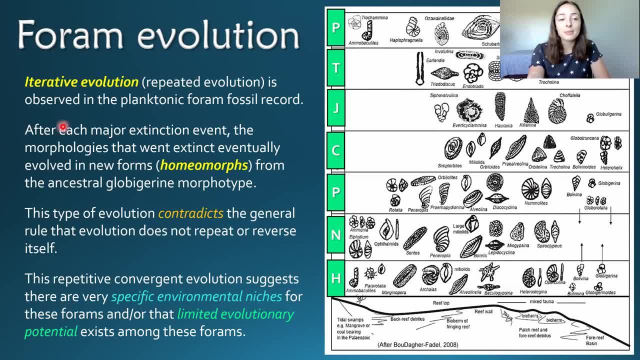 fossil record ever since they evolved in jurassic. what this means is that we see, after each major extinction event diminished their morphological diversity. those morphologies that went extinct eventually evolved in new forms, which are called homeomorphs, when one morphotype or morphology of 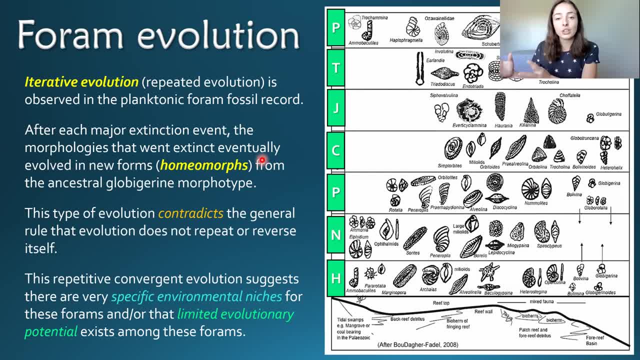 an organism goes extinct, but then it goes extinct and then it goes extinct and then it goes extinct, kind of evolves again in a new form later on in a convergent evolutionary event, because that morphology is beneficial for a certain environmental niche. that new form is called a. 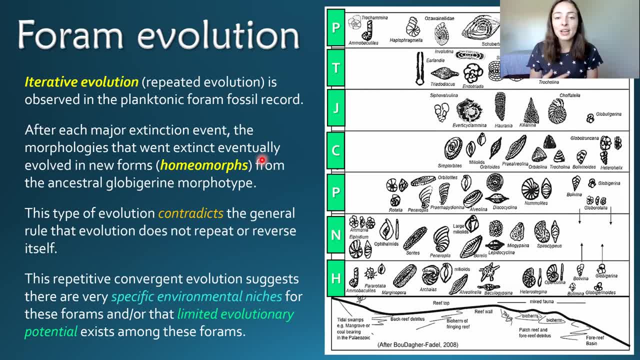 homeomorph and those homeomorphs formed every time these morphologies went extinct from the ancestral globo drain morphotype. they just repeated this pattern after every single major extinction event took them all out. they kept coming back from the simple ancestral type of morphology of planktonic. 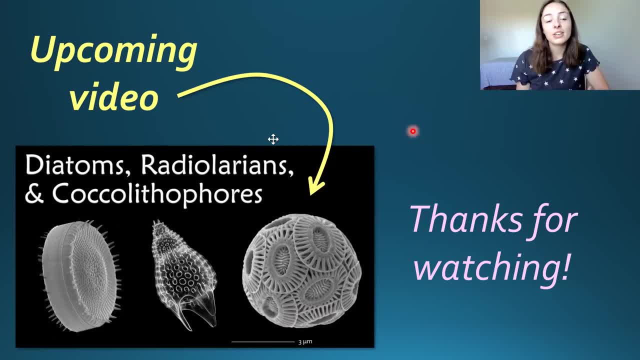 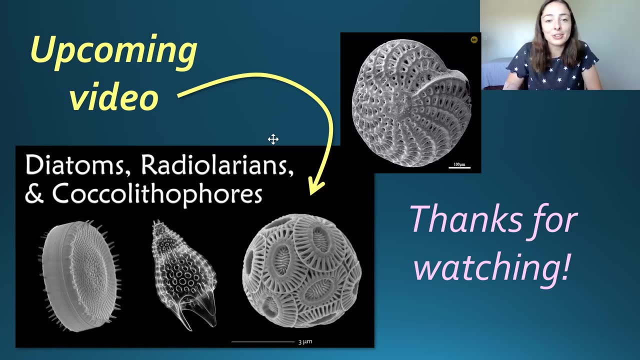 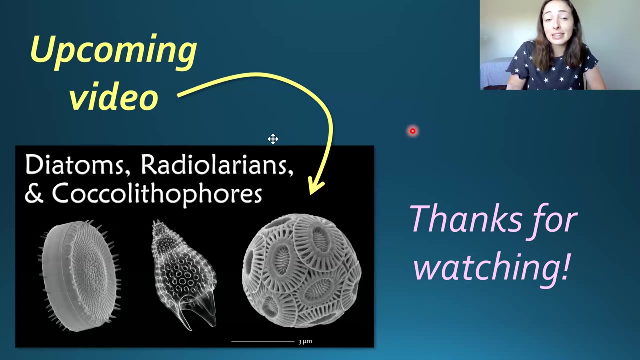 forum, but that is all i have for you guys today. i hope you enjoyed this video. if you did, please give it a thumbs up and subscribe to my channel, if you haven't already, and i'll see you guys in the next video. bye, bye. give a huge shout out to my ta when i took this class, jenny rochelle, who 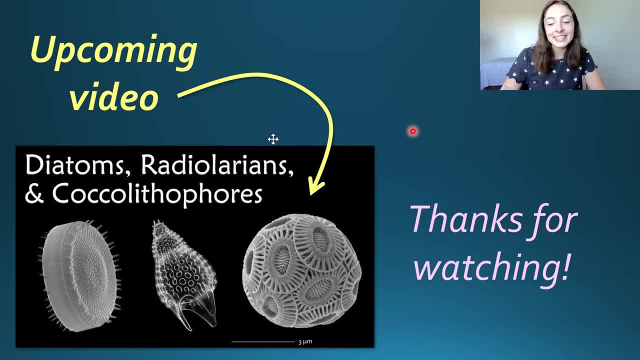 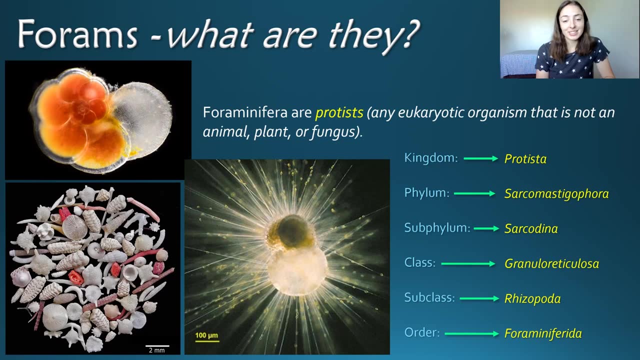 is now a doctor, jenny rochelle, and studies these things like my god. you are such an inspiration, and she gave me a lot of the knowledge that i used to make this video, so shout out to her and, with that, thanks so much for watching and i will see you guys next time. bye, i forgot where i was that. 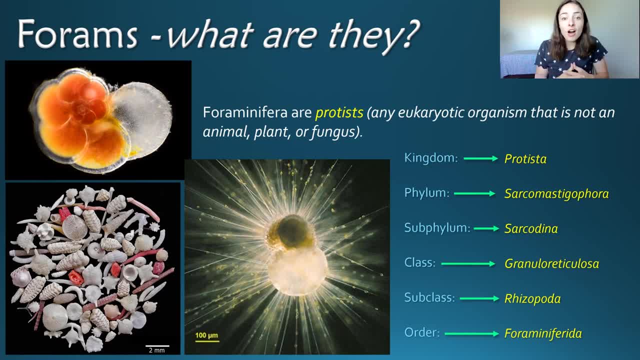 is a problem. sarcomastic aphora. i said that so good, so fast, and i just, I just ruined it by gasping. Rangulo reticuloso, I said that good too. Oh my gosh, Is it Cecil or Cecile, Cecil, Cecile?